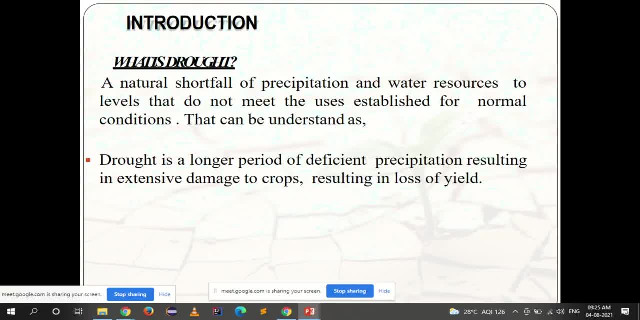 It is a longer period of deficient precipitation. Deficient I mean there is no rainfall or very, very less rainfall for longer period, Okay, Resulting in the extensive damage to crops, resulting in loss of yield. So basically, something that is going to get more damage because of the lack of precipitation. is the damage to crops correct? 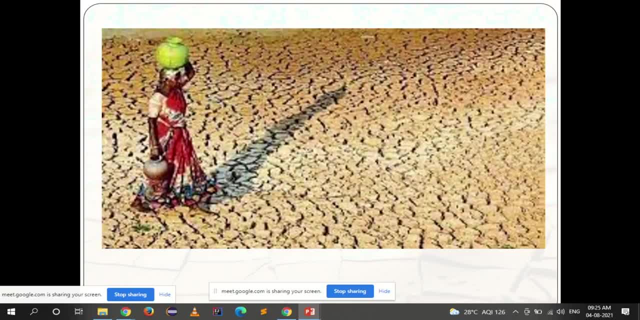 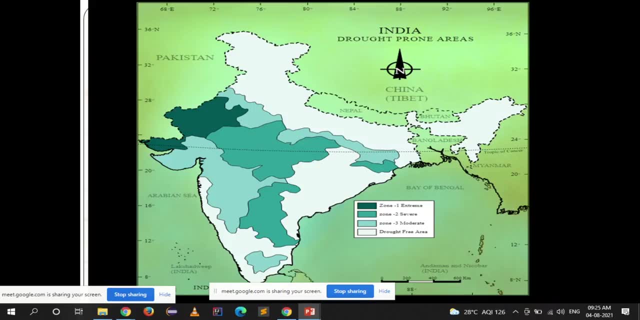 So this is how the drought prone areas look like. when there is no rainfall, no precipitation, The land looks like a barren land, dry, barren land. So this is a drought prone area. So you can see the darker, the greenish color. the more extreme condition of drought is observed in those particular areas. 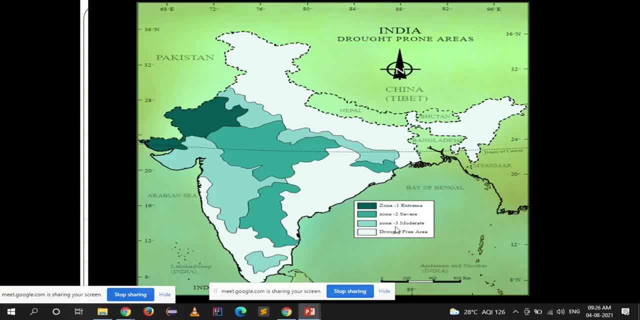 See zone 1, that is, extreme. zone 2, severe. zone 3, moderate and drought free areas are the white colored areas. Okay, So there are. you can say different classification of droughts. So there are. you can say different classification of droughts. 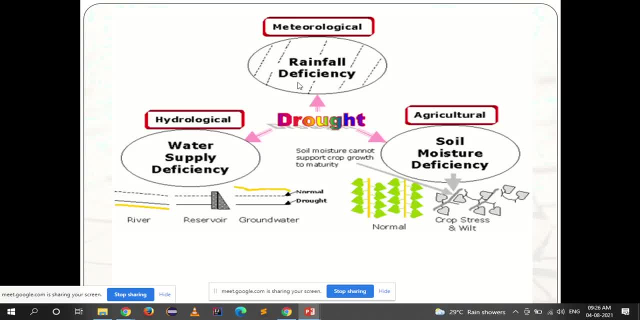 So there are, you can say, different classification of droughts. So depending upon the rainfall deficiency, then soil moisture deficiency and water supply deficiency. So from the diagram itself we can make out, when you talk about meteorological drought, that is drought that is lack of water due to some meteorological condition. that is rainfall. 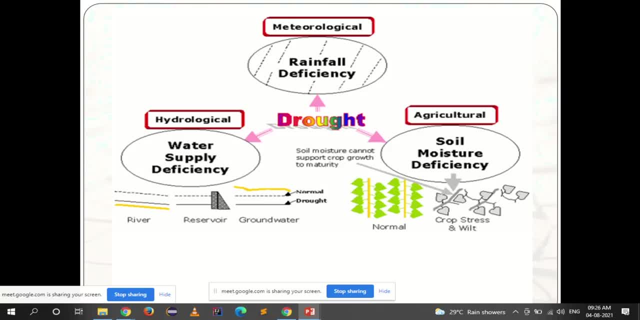 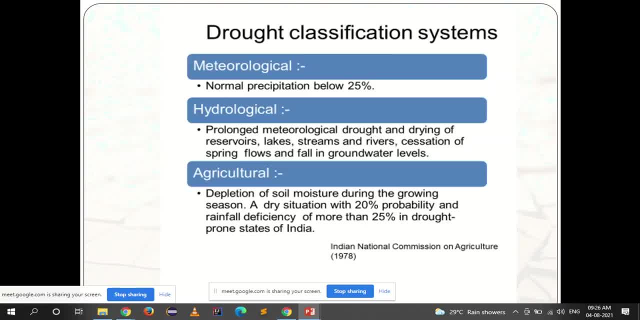 Okay. So if depletion of the soil moisture during the growing season, a dry situation with 20% probability and rainfall deficiency of more than 25% in drought prone states, that is called the agricultural drought Soil moisture. the soil moisture is lost, maybe because of the warm conditions over there. 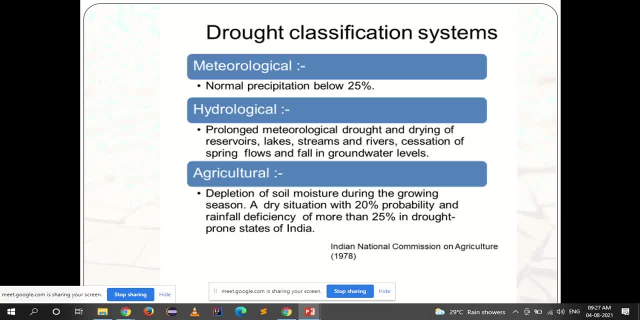 Okay, Okay, Rainfall is one of the reason, And plus the condition there, the area is in such a- you know, a hot climate area that the soil moisture is immediately lost, so that also becomes very difficult for crop to be grown, and that is called the agricultural drought. 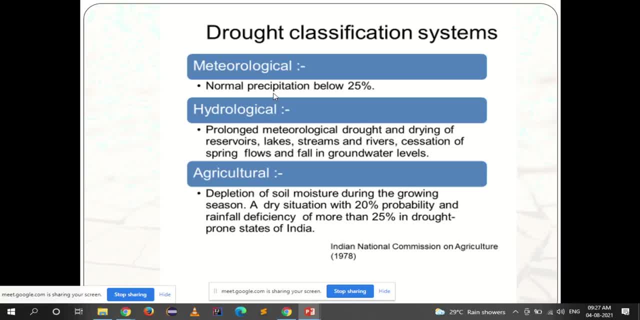 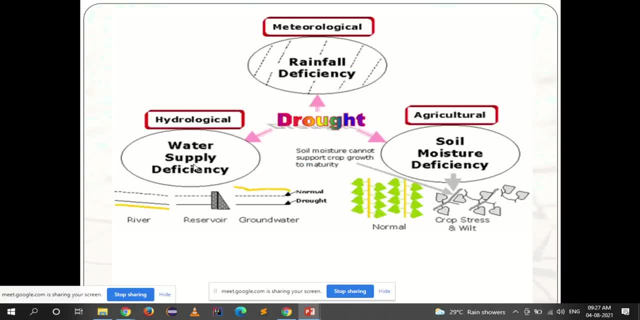 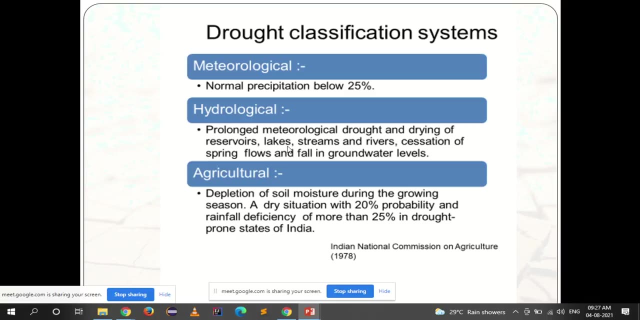 Okay, Meteorological. I just told you that when the rainfall is low, there is normal precipitation below 25%. Okay, Okay, And this hydrological drought, That is, water supply deficiency. So what is that? Prologue meteorological drought and drying of the reservoirs, lakes, streams, rivers, cessation of the spring flows and fall in the groundwater levels. 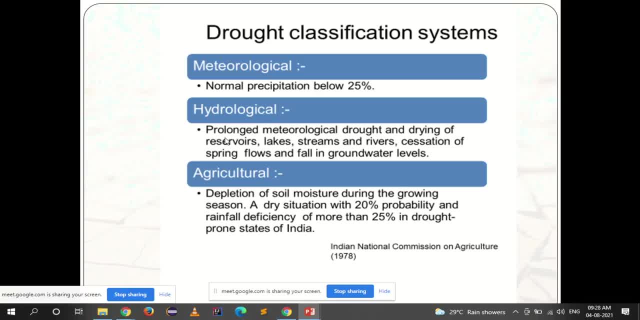 Okay, That is, precipitation is low. Basically, the main reason for drought is low rainfall or no rainfall. Okay, It is related to rainfall, But when it is only related to rainfall, it's called meteorological drought. When it is related to, 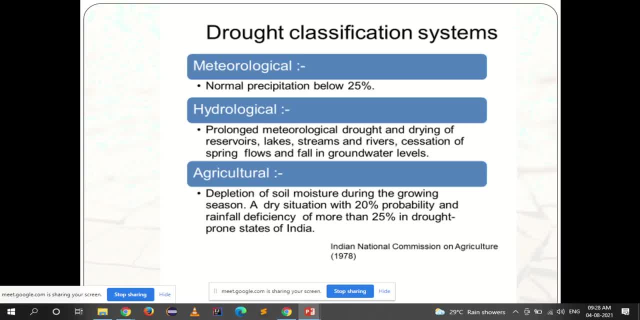 Precipitation, that is, a low rainfall plus drying of the reservoirs, as I told you, if that area is in particular condition, where there is too much hot climate area. so you have drying of reservoirs, lakes, streams, cessation of the spring flows. cessation in the sense, reduction or complete stoppage of the spring flows. spring flow in the sense when the groundwater is high, through different paths to different channels, you can see that there is a lot of precipitation. 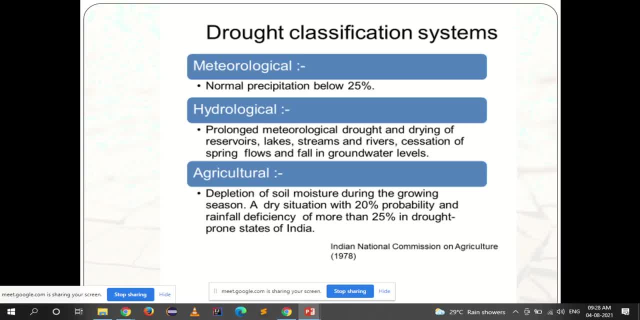 Okay. So, like you have seen the above, in this layer of channels inside the underground, the groundwater reaches the earth surface. Okay, So that channels are called the spring flows. Okay, So stoppage of the spring flow in the groundwater is low. 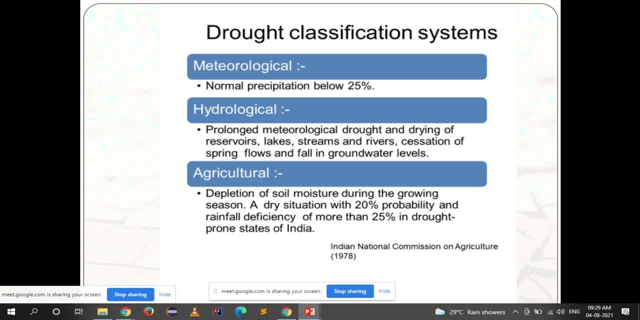 How will you get those spring flows? I mean, how will you get the water rising towards land So that way it also stops and falling in the groundwater levels? Okay, the depression of the soil moisture, along with the less rainfall, of course. okay, then reported. 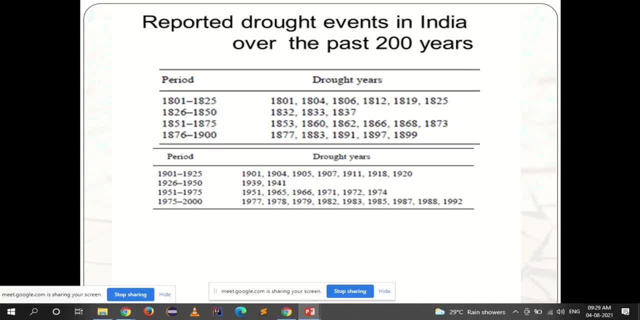 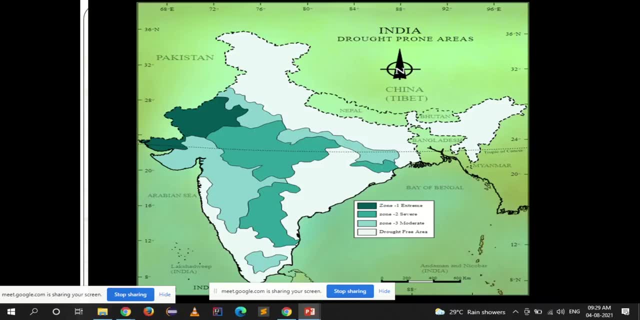 drought events in india over the past 200 years. so these are the actually are. like i told you, like i just shown you the map here you have seen the map. okay, even if extreme drought condition you could see only and to a few places, but still this greener areas are also the drought prone areas. 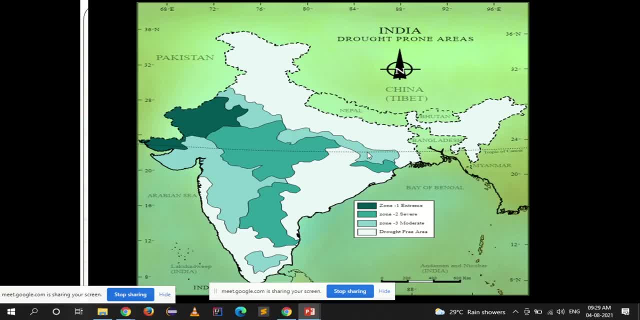 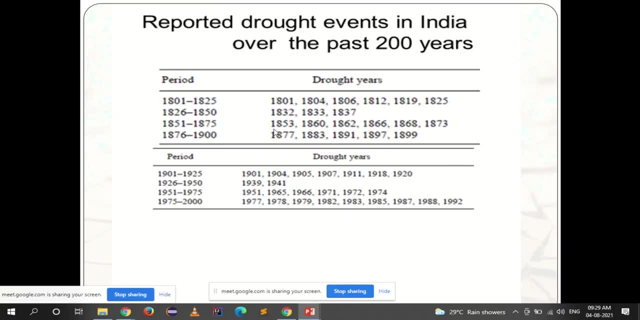 maybe it's a severe, moderate, but still they are in the drought prone areas. okay. so if you look at the map, our country is actually prone to droughts. so you can see the drought years reported drought events in india over the past 200 years, so from period 1801- 1900. so this very drought. 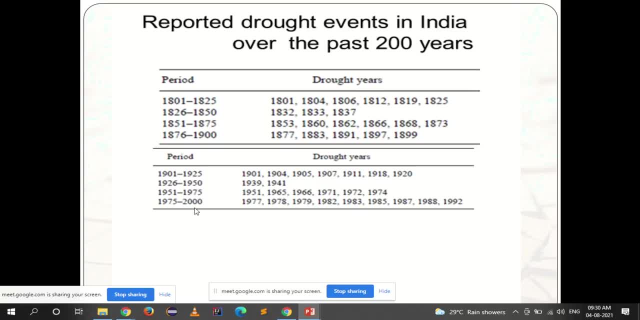 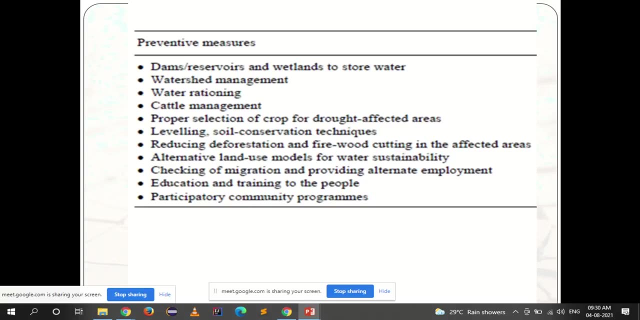 years, similarly 1901 to 2000, so many were the drought years, drought years in the sense. in this years, many parts of the india uh were reported to suffer from drought condition. correct, then? what are the preventive measures that we can follow in order to prevent or, to you know, mitigate, reduce the impact? 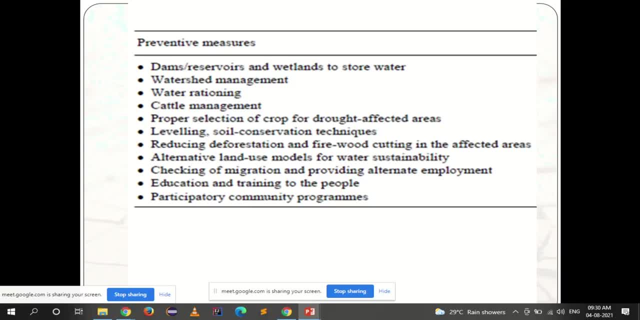 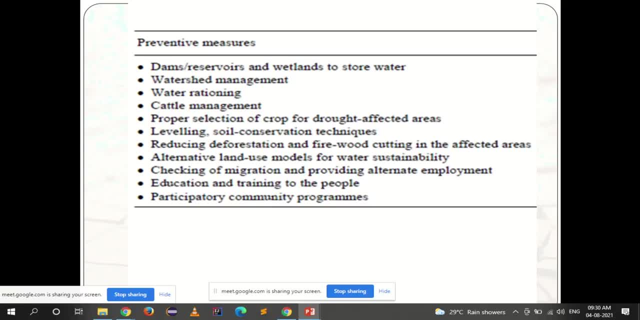 water shade management: wherever there is water is collected- maybe because of the rainfall, maybe because of the streams or the river joining and getting collected somewhere, so whatever, naturally the water is getting collected- management of that water that is collected- that is called the watershed management, water rationing, water ratio lessons. when you have 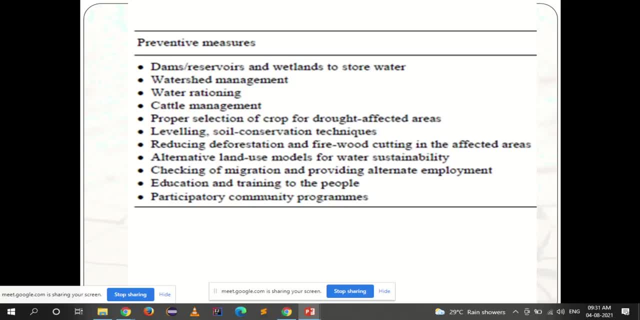 to pay bill for the usage of your water. of course, people using the water, uh people- will not waste the water, right? so water rationing has to be done so that sufficient amount only, adequate and sufficient amount only, will be used by people. cattle management, because when you talk about agriculture, 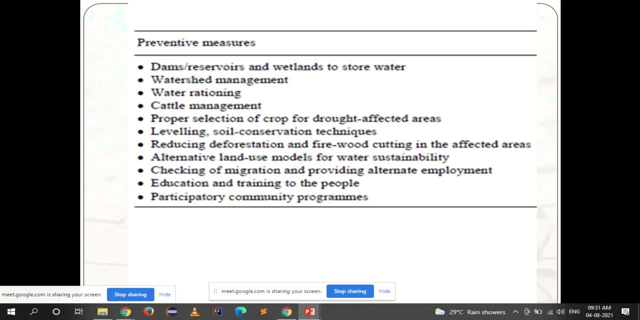 getting much more affected. okay, agriculture and animal husbandry. that is mostly for the crop- uh growing, uh growing of the crops- as well as to the, the farmers having their animals, because they also require water in this drought prone areas. it is very difficult for them to survive. okay, so cattle. 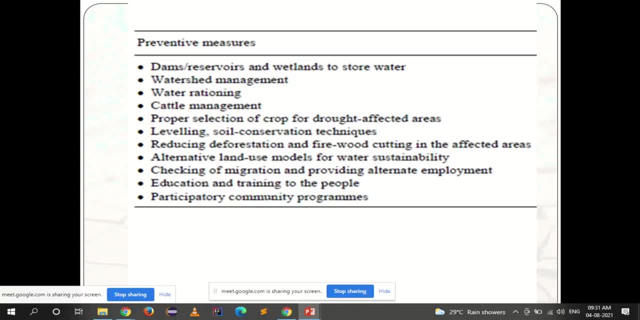 management, proper selection of the crop for drought affected areas. okay, so that has to be done. then leveling and soil conservation technique. how you can have, uh, what you say: the more amount of soil that is permeable. so, the more amount of soil that is permeable, the more amount of soil that is. permeable. if the soil is permeable, it will absorb a lot amount of rainfall, correct, and it will increase the groundwater level. it will always be moistened then, reducing deforestation and firewood cutting in the affected areas, because that is one of the reason which increases the temperature of. 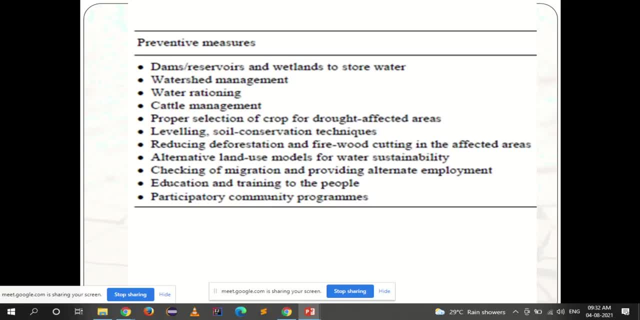 any area, correct? so reducing deforestation so that the climate will not be a hot climate, more hotter climate, basically, if it is in the hot prone area, but more hotter, uh, it shouldn't happen. so that could be reduced. uh, that could happen by reducing deforestation. firewood cutting in the affected areas, alternative land use models for water. 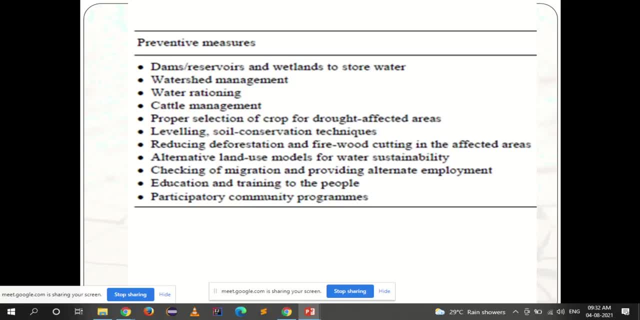 sustainability, how you can use the land in such a way that water could be used in only adequate amount. then checking of migration and providing alternate employment. if, in the drought prone areas, people- basically when farmers- are faced with a lot of problems, how you can provide them alternate employment in those particular. 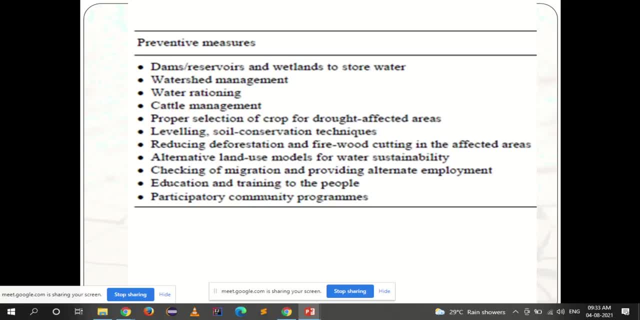 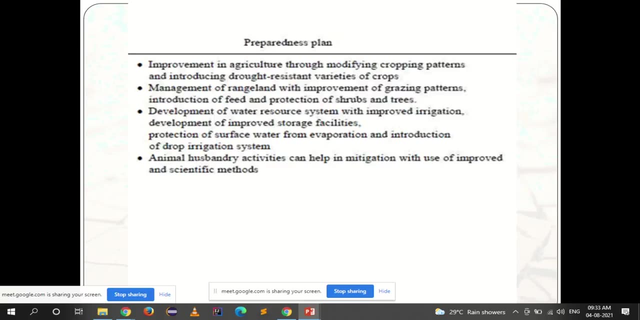 uh, years, or what do you say? period of time when there is drought, education and training to the people to be given on how to face this drought, and participatory community programs, so all these preventive measures can be followed in the drought prone areas, then preparedness plan, improvement in. 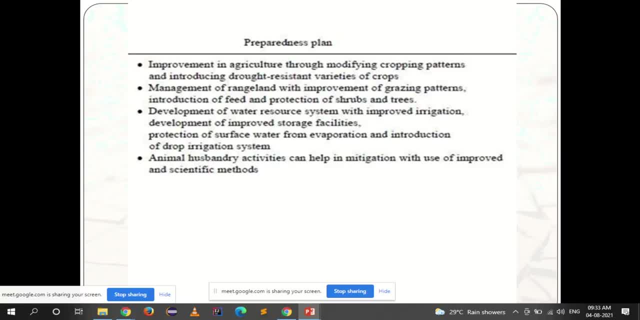 agriculture through modifying the cropping patterns and introducing broad resistant varieties of crops. just i told you that you can change the crop patterns more and then more of using of broad resistant areas in those period of drought. then management of rangeland, with improvement of grazing patterns, introduction of feed and protection of the shrubs and trees, development of water resource. 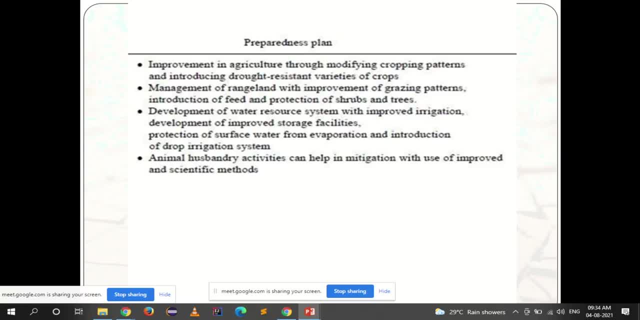 system with improved irrigation, development of improved storage, water storage facilities, protection andlax suti on garden soil in general, bottom and surface water from evaporation and introduction of drop irrigation system. so all these things can be followed in relation because, like just now, we have seen the type of growth along with the precipitation. it is the hot climate also. 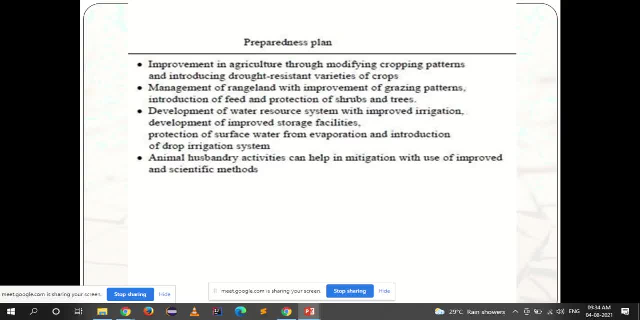 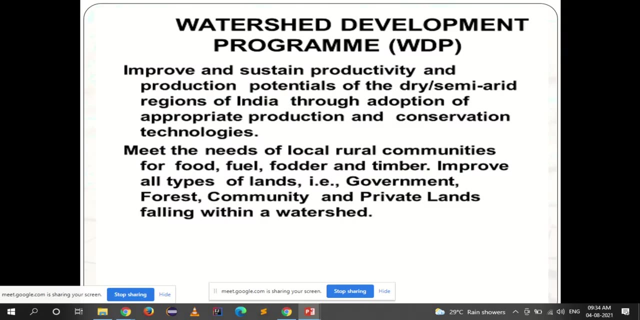 in that particular area, which are the main reasons. so that is where you have to protect the surface water from evaporation. then introduction to drip irrigation system. actually it is then animal husbandry activities can help in mitigation. scientific methods, then watershed development program. watershed development program in the sense, like I just told you, when we talk about 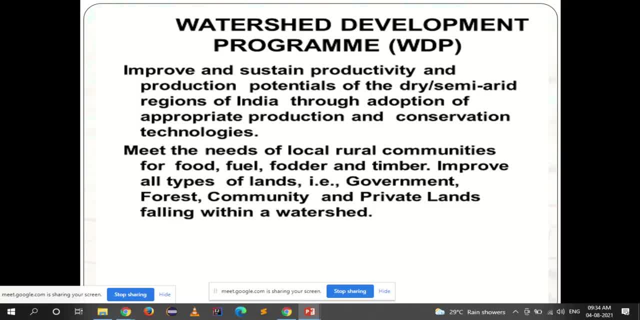 watershed management. it is amount of water that is getting stored naturally in a particular area, getting collected. so how to manage that? how to, you know, preserve that, so improve and sustain productivity in, and production potentials of dry and semi-arid regions of India through adoption of appropriate 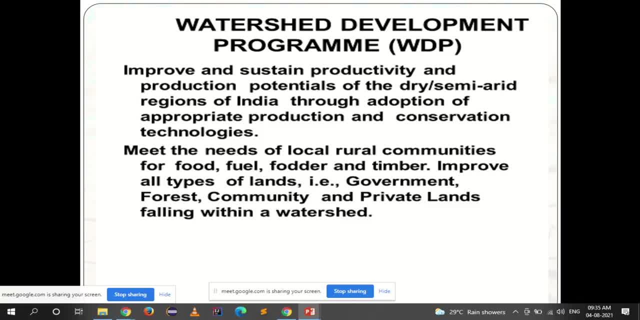 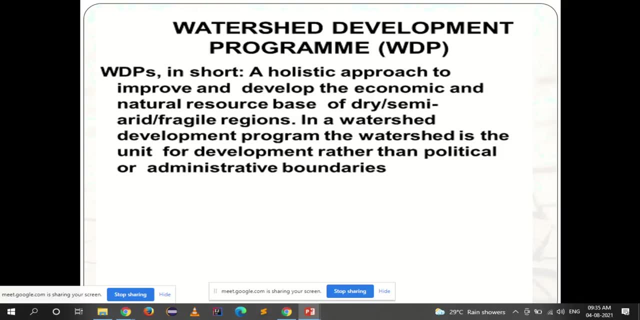 production and conservation technologies. meet the needs of local rural communities for food, fuel, fodder and timber. improve all types of land, that is, government, forest, community, private lands falling within a watershed. then what is this watershed development program? it is a holistic, a complete operation of the watershed development program. it is a holistic, a complete. 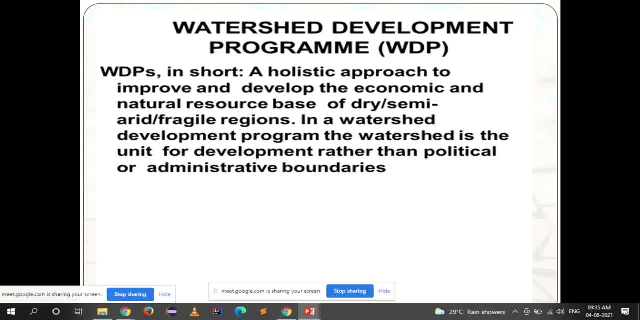 operation of the watershed development program. it is a holistic, a complete approach to improve and develop the economic and natural resource base of dry or semi-arid or fragile regions. in a watershed development program, the watershed is a unit for development rather than political, administrative boundaries. the more and more the water can be collected, like now. you see the 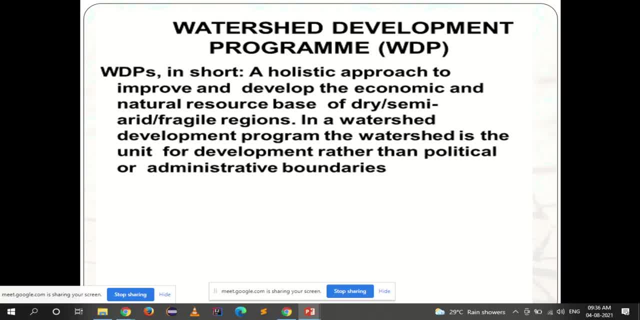 work of Pani Foundation. you can, you might be a part of it, your relatives might be a part of it, or some known person might be a part of it, or you have seen it on the news, also on your television also. then how in that Pani Foundation in rural? 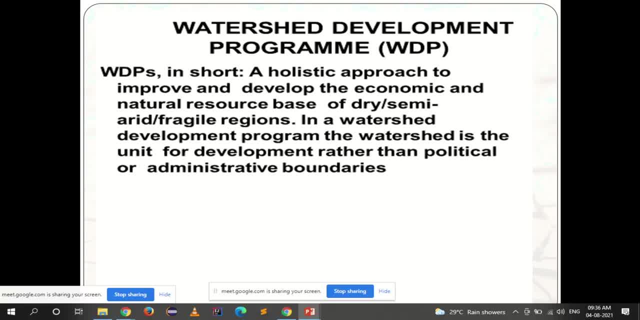 areas, basically, where people, where the main source of income of people is agriculture and we are more dependent on water. for it, of course, water is the main source for it, and when they they face this lack of shortage of rainfall, then how they come together and help in storage of the water. how much ever water is received, we don't have to. 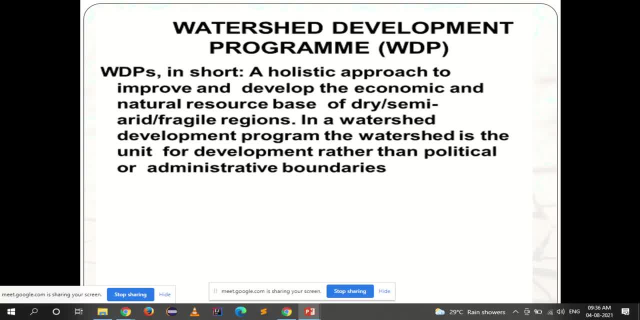 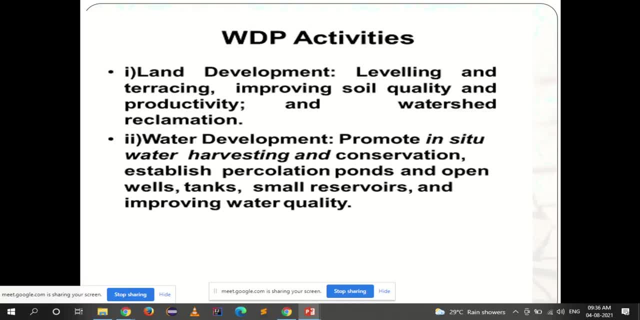 waste the water. we have to manage that water, preserve the how much of the water that is received. so that is actually comes under the watershed development program. see what are the different watershed development activities: land development, leveling and terracing, improving the soil quality and introduction and productivity and watershed reclamation. okay, then water. 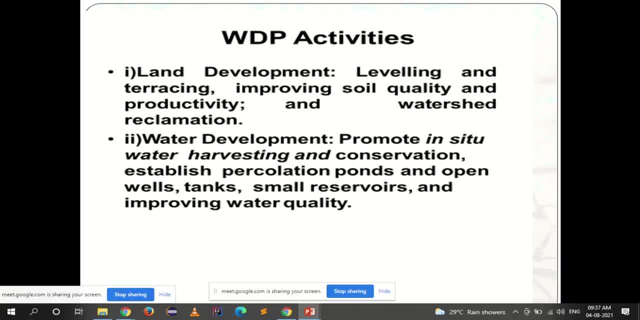 development promote in situ on the site: water harvesting, conservation, established percolation ponds and open waste tanks, small reservoirs and improving the water quality. so all this comes under the WDP, that is, watershed development program activities. okay, land development, that is leveling, terracing, I mean, why do you have to do that so that the surface runoff? the 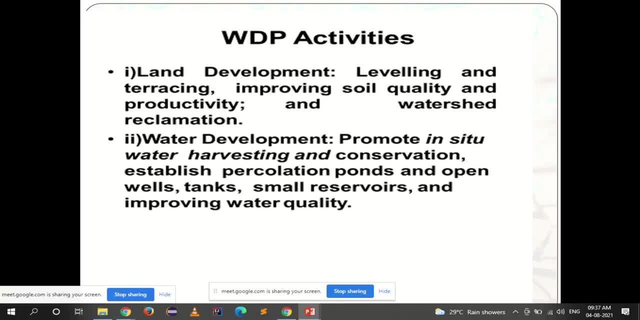 water that is received should not get runoff, should get percolated inside that soil, okay, and therefore you have to do this. leveling, okay, we should improving the soil quality so that, like I said, permeable soil we need. then watershed reclamation: again, we are improving the watershed areas more and 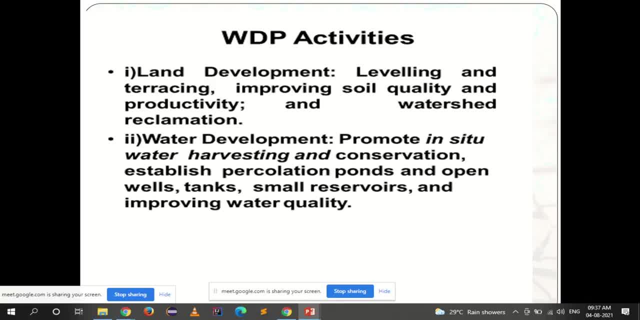 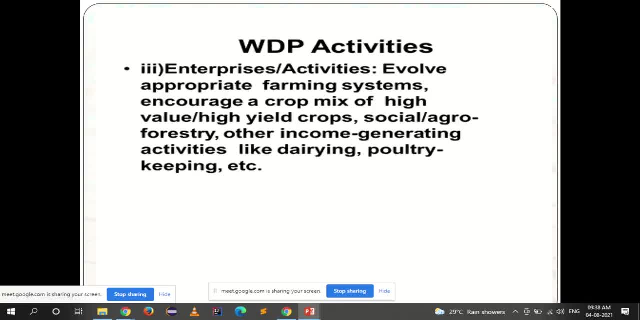 more water that could be stored, then water harvesting, conservation of percolation, open well tanks, small reservoirs and also improving the water quality- all this comes under watershed development program activities, then natural that is evil. appropriate farming system, encourage a crop mix of high value and high yield crops, then so she and a grow forestry and other income. 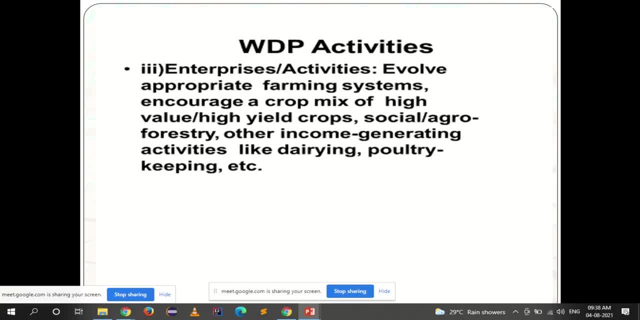 generating activities, like I said, not only on the single income, when this particular session is observed in that area session of people should be made away, or with different income generating activities also, and how the modern techniques or, uh, what patterns could be followed. different modern patterns could be followed in the 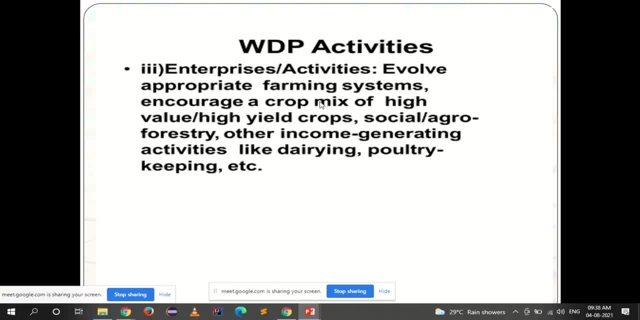 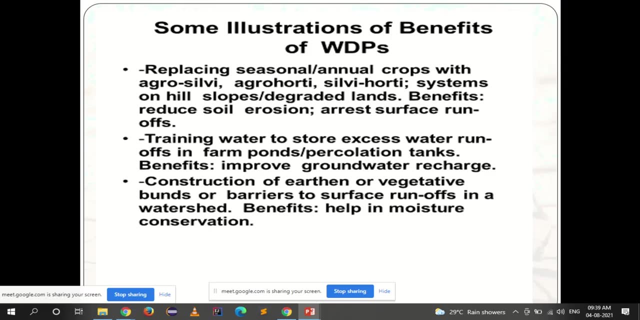 agriculture and land use system. okay, like here it is given. encourage the crop mix of high value, higher crops, okay. so all these activities need to be followed and need to be made people educated about it. some illustrations of examples of benefits of watershed development programs: that is, replacing the seasonal or annual crops with agro sylvie, agro horty or sylvie horty. 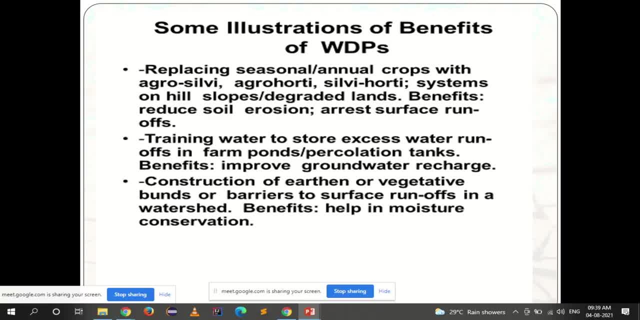 systems on hill slopes or degraded lands. that is benefits are: it reduces the soil erosion and arrest the surface runoff. okay, so, like we were talking about, that is, uh, the crop patterns, the land use pattern, the type of crops that are being used. okay, that has to be. 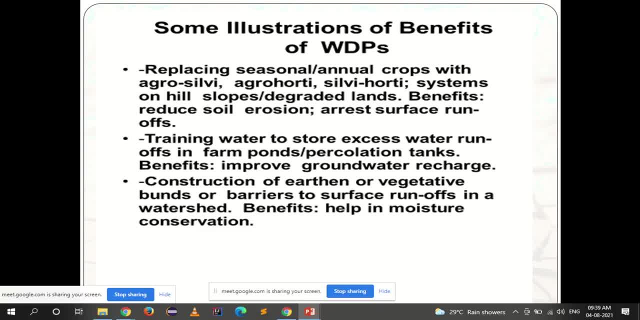 changed correct. so, replacing the seasonal or annual crops, let's just open up. so, when you talk about use, uh, replacing the seasonal or, uh, this, annual crops, which are normally being, uh, you know, grown in that area, with agro sylvie, agro sylvie, in essence, there are certain plants which grow in the forest areas only. so those are. 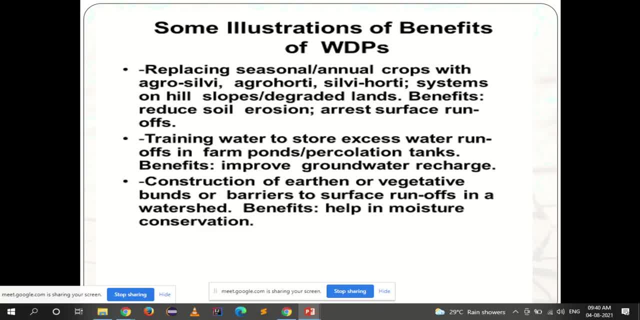 called the sylvie crops, forest areas. so, just having the agricultural crops, you can replace it with mix of agro and forest crops, mix of agro and horty. agro, horty, horty, you know, plants, or, um, what you say, food based crops, uh sorry. 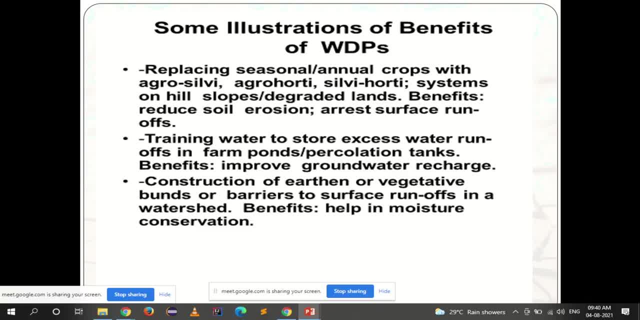 plants. okay, so you can have agriculture crops and plus you can have flowers or food- uh, food based plants, then sylvie horty. there is forest sylvie in the sense when you talk about the plant based crops. in the sense, we have a lot of the that are grown in the forest horty in the 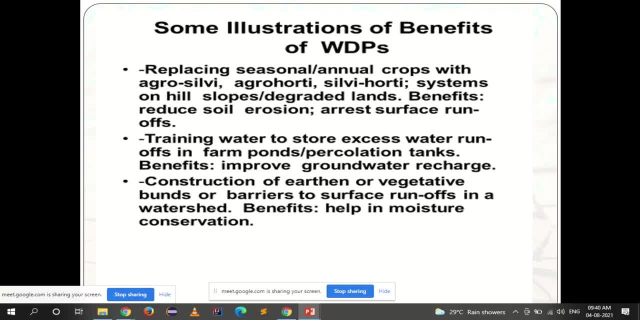 sense animal or the plant-based plants. so you can have that combination, okay, all systems on hill slope and degraded lands and benefits. it reduces soil erosion and erase the surface runoff. like i said in the previous slide itself, you have to arrest that surface runoff. i raised innocence. 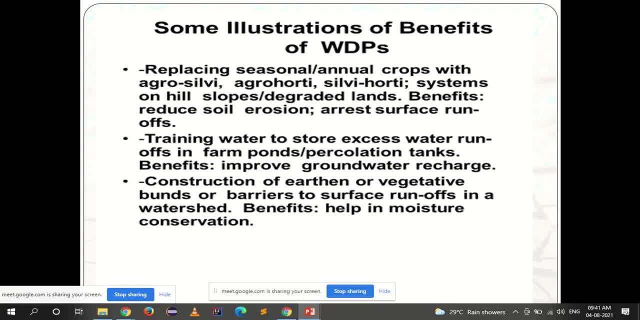 because of the surface level of course you have. you cannot change completely the topography of if that particular area is in the sloping region because of the rainfall, whatever short rainfall you get, no water will be arrested because it will get runoff from the sloping area and plus. 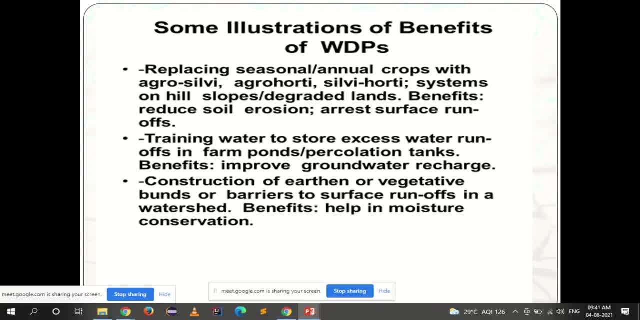 because of that runoff, the soil erosion will happen, which we don't want, because we want soil to be present there so that ground water could be increased by the absorption of the soil. so that is why you have to have the crops grown on this sloping area, which will erase the surface. 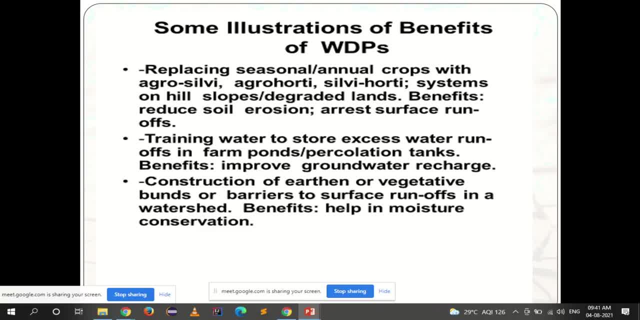 you know, okay, and you should absorb the more amount of water. okay, then, draining water to store excess water runoff in farm ponds or percolation tanks benefits, that is, improve the groundwater recharge. okay, farm ponds, percolation tank, where it will be stored and it will be you know. 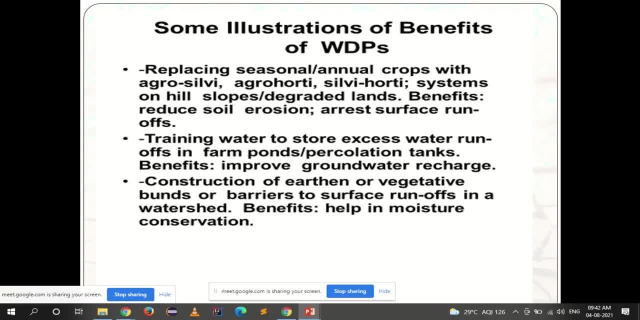 go through through the soil and increase the groundwater recharge. construction of the earthen or vegetative bunds or barriers to surface runoff in watershed. wherever there is surface runoff, wherever the water is flowing through the slope, like we said, that is growing of the crop. i mean the different types of crops that will arrest the surface runoff, or you can have 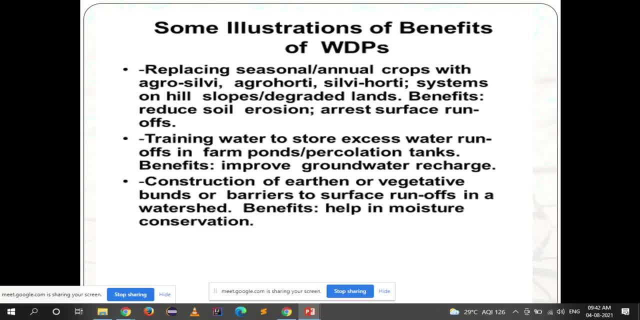 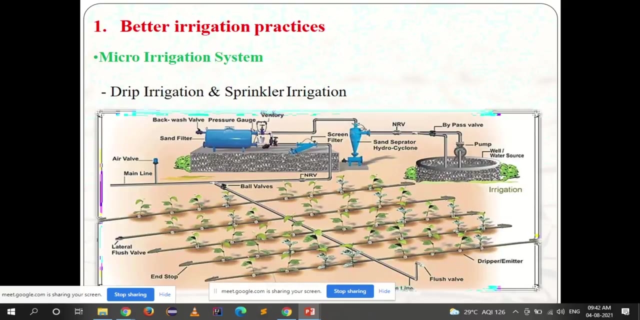 construction of the barriers, the bunds. like i told you, bunds are also this small barriers, only barriers, which can erase this surface and collect the water. it helps in moisture conservation. okay, so this way's few of the examples that could be uh followed and what resource management in brought from the figures or what you said, from the images we can see. 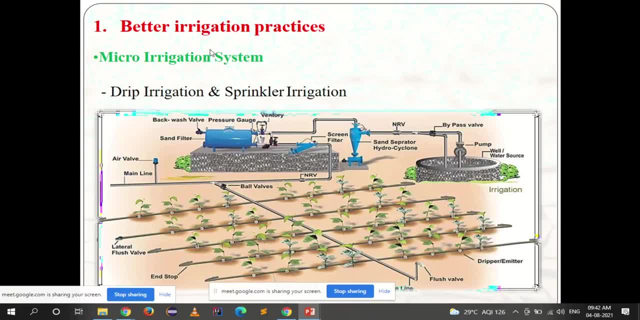 see this: better irrigation practices: micro irrigation, drip and sprinkler irrigation- you must have studied this at your cool level as well- directly usage of water, rather than having this drip and sprinkler irrigation which uses sufficient amount and adequate amount of water only so that has to be followed in the 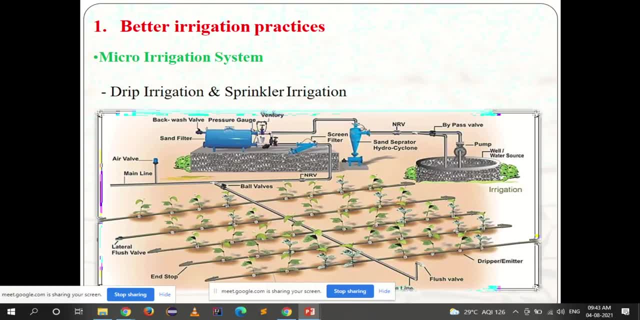 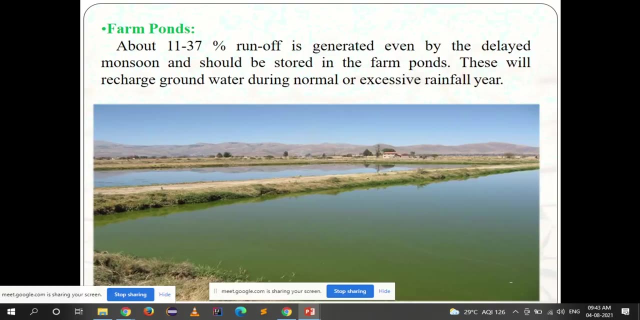 areas, which is in the drought prone area, so that the wastage of water, unnecessary wastage of the water, could be reduced. an adequate amount of water will be available through this type of irrigation system. correct then farm ponds. about 11 to 37 percent runoff is generated, even by the 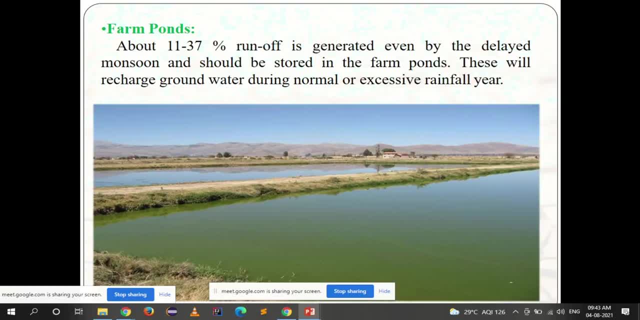 delayed monsoon and should be stored in the farm ponds. this will recharge the groundwater during normal or excessive rainfall year. understood? that is what i was talking about, the pani foundation work also. so it is somewhat. it is a similar type, that is, when you are creating ponds in your farm itself, those are not. i mean you don't have to construct. 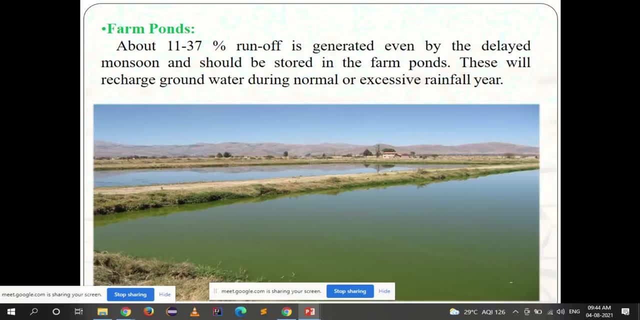 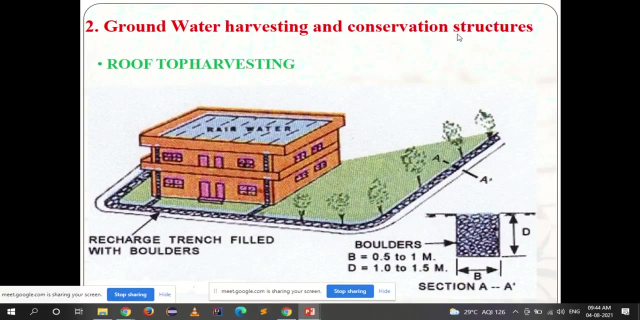 anything. you are just creating ponds so that, if the water could be stored, the groundwater recharge could be increased. okay, so that are called the farm ponds. that also comes under this: better irrigation practices, groundwater harvesting and conservation structure: conservation structures. so for that, rooftop harvesting, rainwater harvesting, correct, so you know this- when you have sufficient area, which we call the catchment. 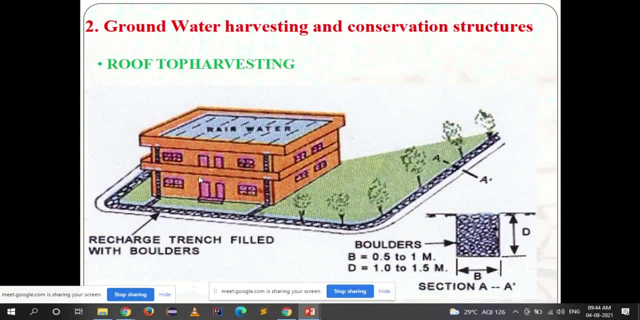 area. now this for this particular- uh, what do you say? a bungalow or a building, this particular rooftop is the catchment area area which directly catches the water. okay, so the catchment area is so much and this water, rather than getting wasted out, it could be used up. 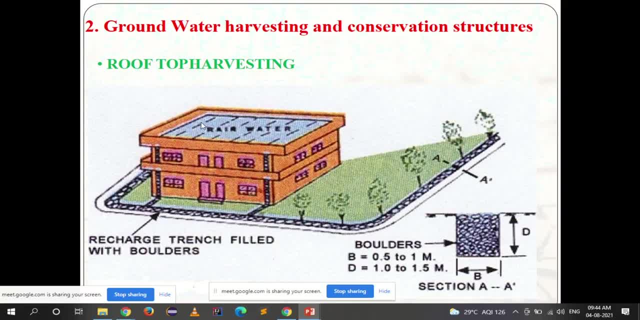 would be used to bring the rainwater to the trendy soil. so the river under the roof of groundwater has been遠ристed, but with these solutions which led to this for the water quality, such as the temperature, and say, moving water fully into the ponds or not, 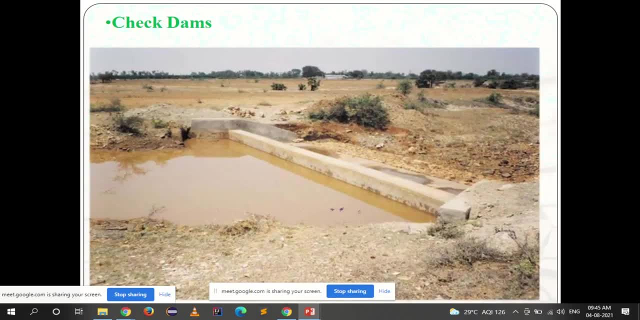 by adding small globalListen, such as the wind turbine housing, or by using linear programming, or if you are using Aldpaper to collect groundwater. we are using such systems for kind of ourjections Check dams, like you had farm ponds. similarly, when you construct, see, this is now constructed. 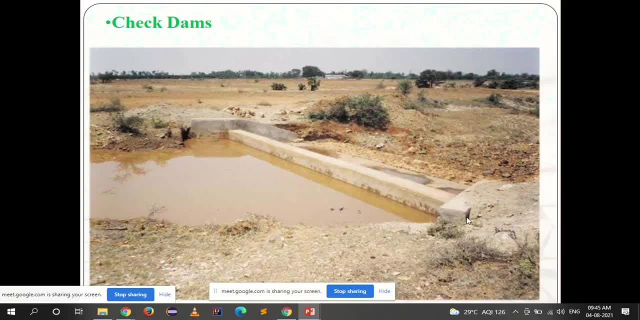 one when you construct the barrier in order to store the water. that is called the check dams, ok, not the regular type of dams, ok, it is just the small barriers that are constructed in order to store that water and avoid the flow of water. percolation times- correct, see. 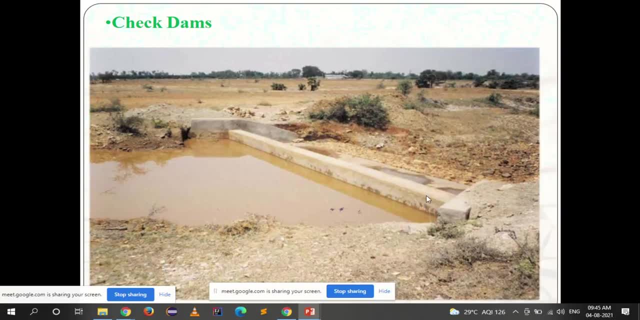 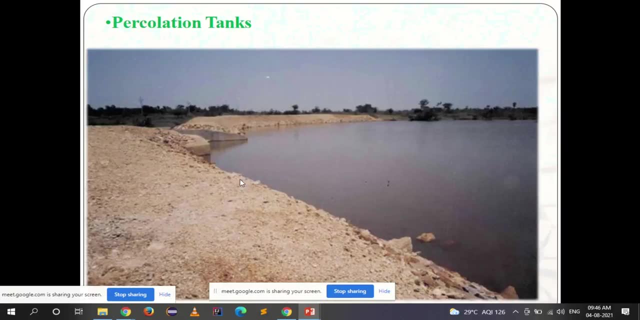 it is just that in this check dams you had a constructed barrier. artificially constructed barrier, I mean using the construction materials, and here it is similar like your farm ponds, but farm ponds are the ponds made in the farm itself so that that water could be directly used for agriculture. 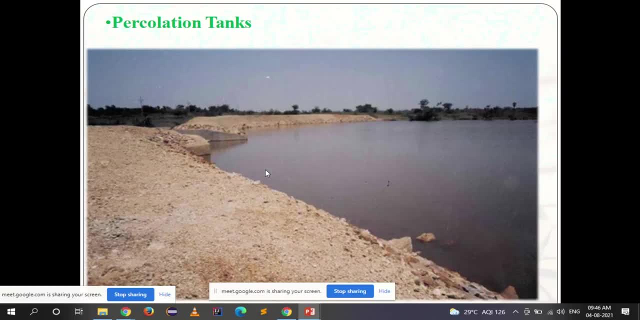 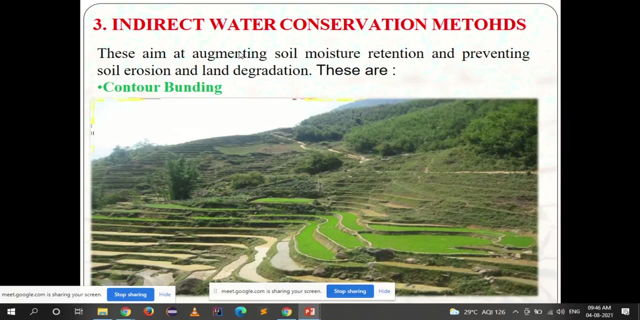 Here very much. it is similar to the ponds that are made in the farm itself so that the water could be collected in that area. percolation times like a lake only could be created. Then indirect water conservation techniques. what are the different indirect water conservation techniques? this aim at augmenting the soil moisture retention- ok, holding the soil moisture. 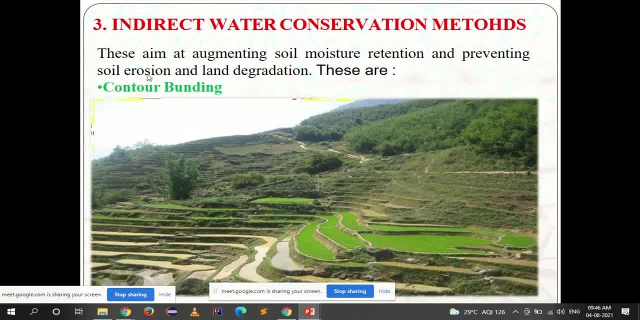 and preventing the soil erosion and land degradation. Now, if you see here This particular area is a slopey area. ok, if there are no counter this contour bunding- that is called contour bunding- if not done here directly, the precipitation, that is, the rainfall that is that falls over this land, then will be a surface runoff and the water. 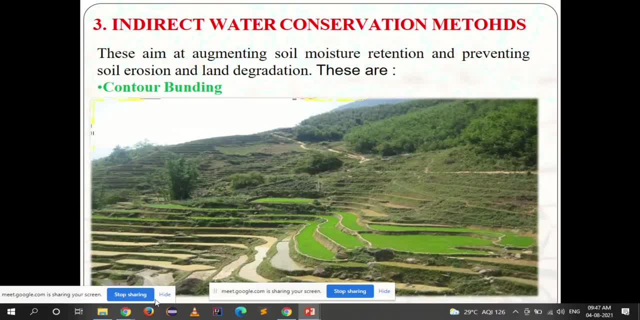 won't be collected in that area, ok, and that will also reduce the soil moisture. of course you have plants here, But still, in order to increase the soil moisture, So you have to keep the soil moisture, So you have to keep the soil moisture. 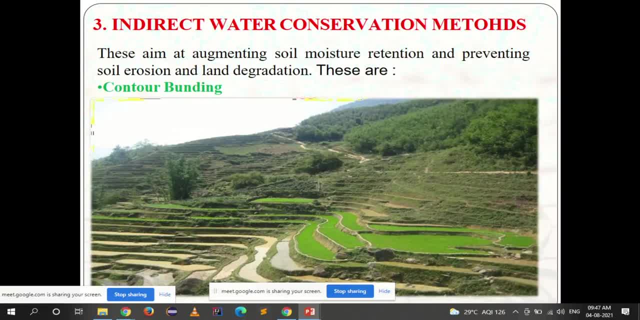 with extension and, on word, soil erosion which happens into the surface, runoff this contour, bunching. the new, You know, construct this bunch Or this slope areas. Of course water will fall through this area, but much of the water would be collected if you see your. 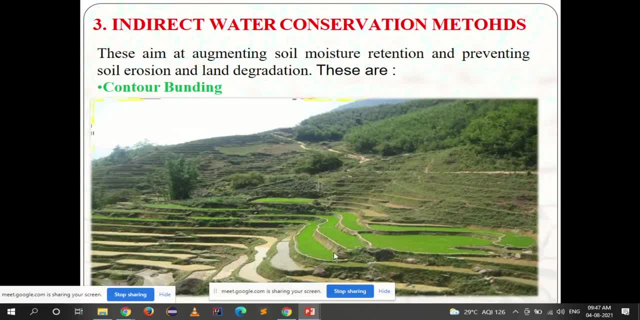 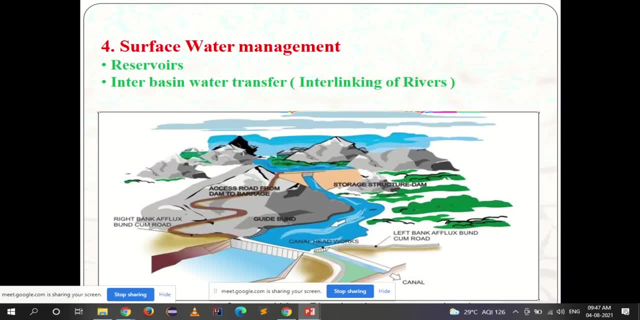 Much of the water would be collected inside this And much of the retention- Okay, really, things now que'd moisture- will happen. Correct, 2.. correct then, surface water management, that is reservoirs. inter basin water transfer, that is interlinking of the river, so that the river interlinks and then goes into some portion. 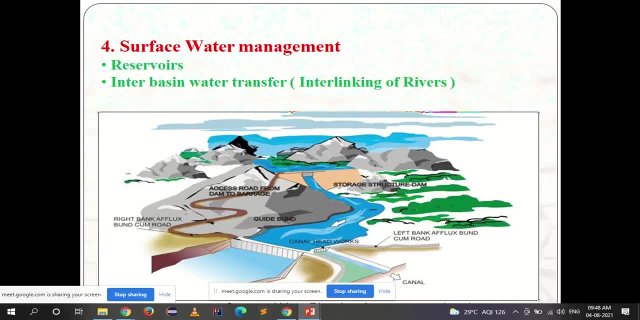 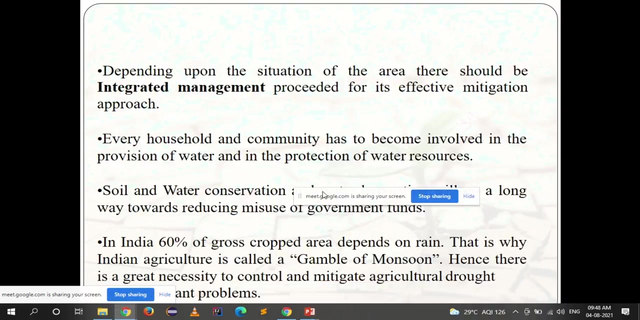 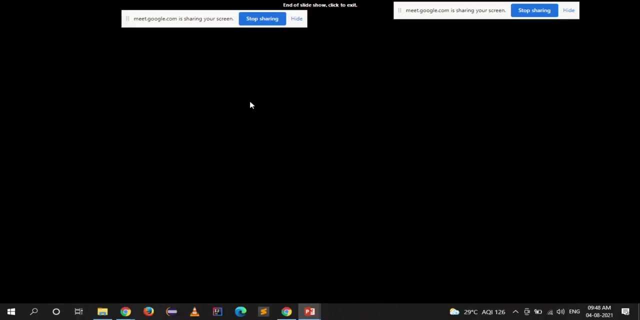 or gets wasted somewhere, or i mean it has to be transferred in order that that water, without getting wasted, it could be stored okay. so you see, here the bunds are made, the canals are made so that the water could be diverted and stored okay there, depending upon the situation. 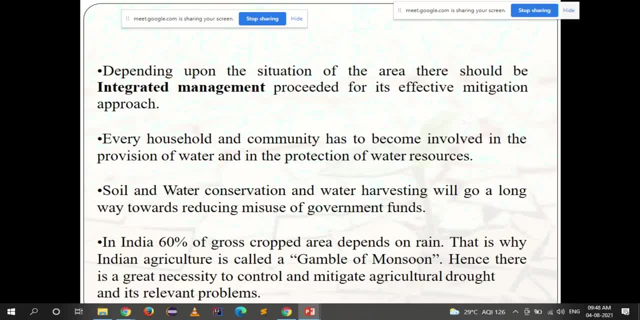 of the sorry. depending upon the situation of the area, there should be integrated management procedure for its effective mitigation approach. right, we have now seen so many things that could be followed for management, management, management of the watershed. so, depending on the situation of the area, the best practices could be followed. 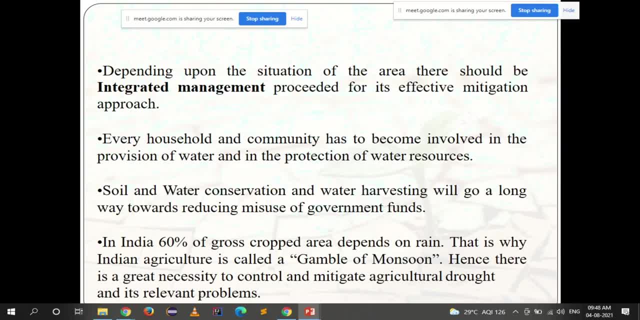 every household and community has to become involved in the provision of the water and in the protection of the water resources, and that is the main motto of any foundation. also, every household, every community should come together and help in this water conservation. soil and water conservation and water harvesting will go a long way towards reducing the misuse of. 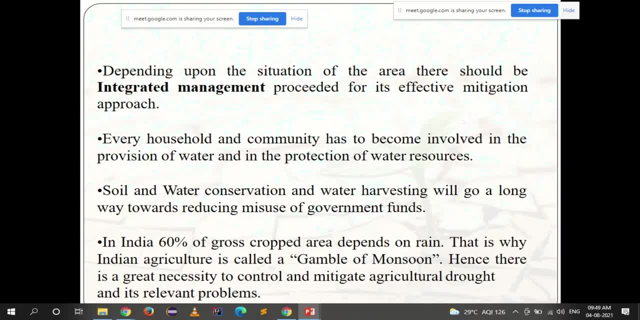 the government funds. soil and water preservation will go a long way towards reducing the misuse of the government funds. soil and water conservation and water conservation will go a long way towards reducing the misuse of the government funds. soil and water conservation and water conservation will go a long way towards reducing the misuse of the government funds. 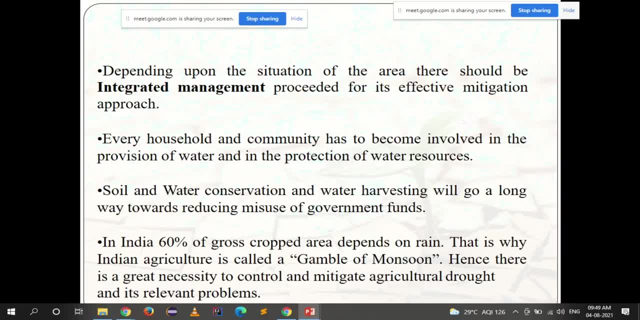 right, right right. in india, 60 percent of the grass이랑 müsste, in india sixty percent of the grass. Итак, india To control and mitigate the the. that is why we have struggle more in this particular field in order to control and mitigate the. 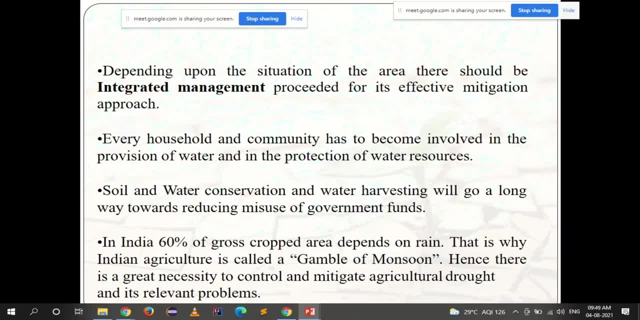 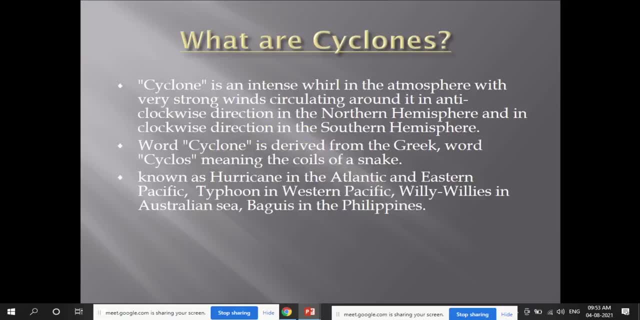 the relevant problems, right. so we work like this: keep measuring water redemption and managing, inom the agreement to manage the problem of the uh flood water against the relevant problems, rightý. so the next disaster that we will go through is cyclone. okay, so what are cyclones? cyclones. 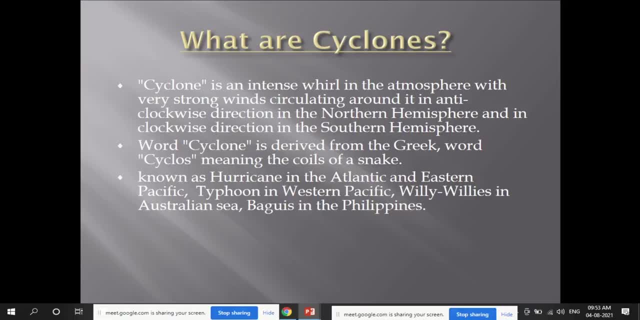 we had seen, we had heard about it, we have seen in the videos as well. okay, so cyclone is an intense whirl, okay, the churning or turning around. okay, so it is an intense whirl in the atmosphere, with very strong winds circulating around it in anti-clockwise direction in the northern hemisphere. 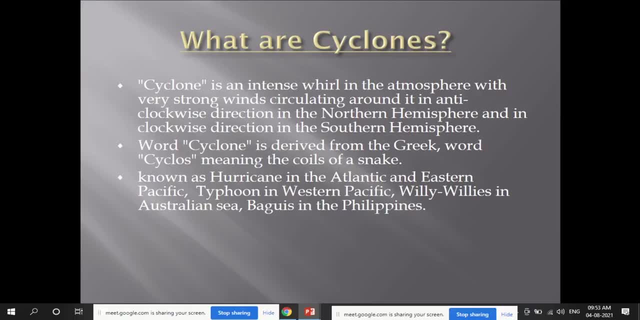 and clockwise direction in the southern hemisphere. okay, so it are the intense whirl in the atmosphere, intense whirl of what? the strong winds circulating in anti-clockwise direction in northern hemisphere and clockwise direction in the southern hemisphere. the word cyclone is derived from the greek word, which means cyclose, which is a cyclose word, and 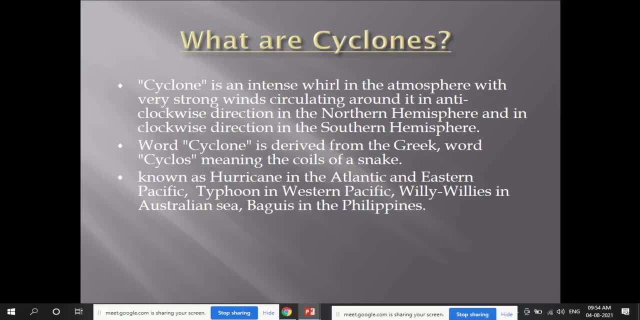 the meaning of is is coils of a snake. so how it is? the coils of the snake are whirl around the similar is the cyclone, and that is why. that is why the word cyclone was derived from this word cyclose. now this cyclone has different naming at different places, so it is known as hurricane. 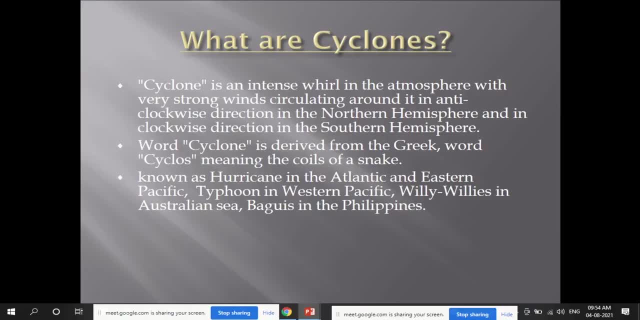 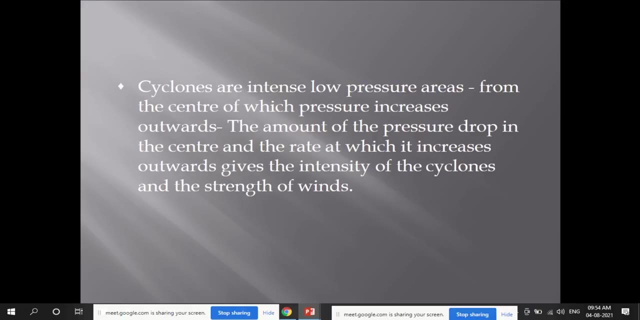 in the atlantic and eastern pacific, typhoon in the western pacific, willy willies in australian sea and buggies in the philippines. so it is one and the same, but it has different names at different places. then cyclones are intense low pressure areas from the center of which pressure increases. 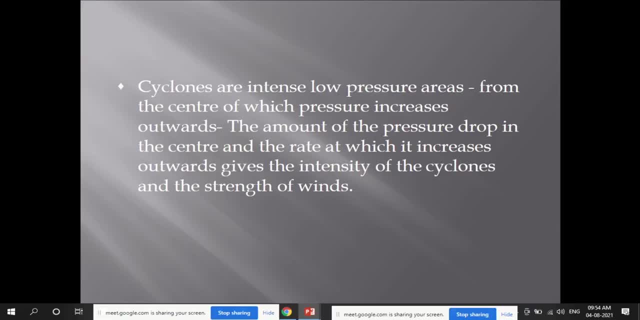 outwards. the amount of pressure drop in the center and the rate at which it increases outwards gives the intensity of the cyclone and the strength of the wind. okay, it is the low pressure area at the center and high pressure area at the center of the cyclone. okay, so 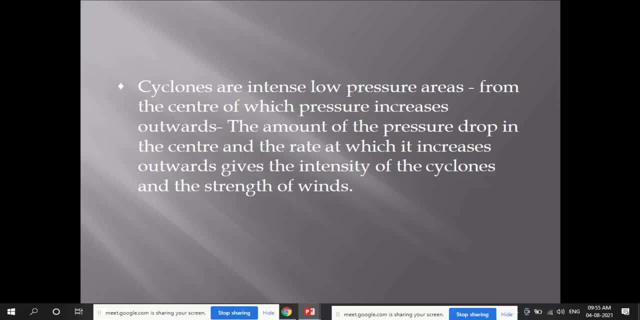 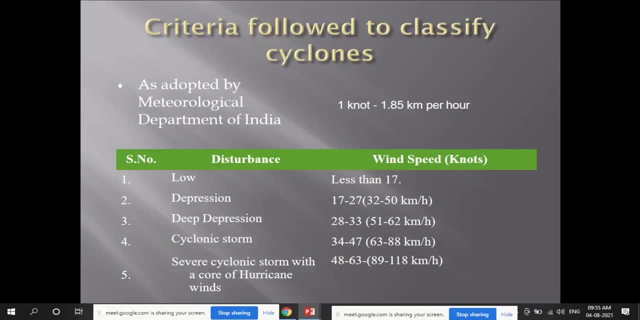 the center and high pressure area at the side. okay, so the center of of which the pressure increases outwards. okay now, because i didn't have to- also to classify the cyclone. when you say low deep, i mean depression, depression and cyclonic storm, severe cyclonic storm with. 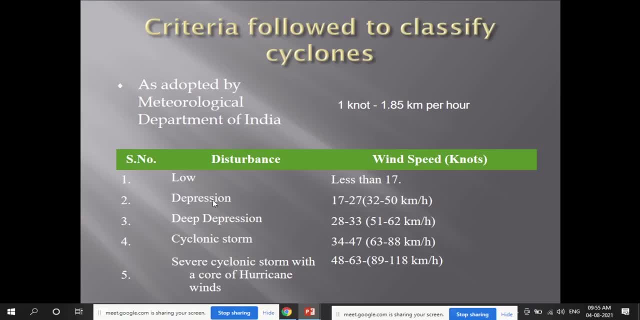 a poor of hurricane mans pottery class Castle is classified based on the wind speed because, like i said, 10 and 16- it is a bird舩의 windcrap- is classified. it is classified based on the- Like I said, it is the whirl of the wind and the fast moving wind. 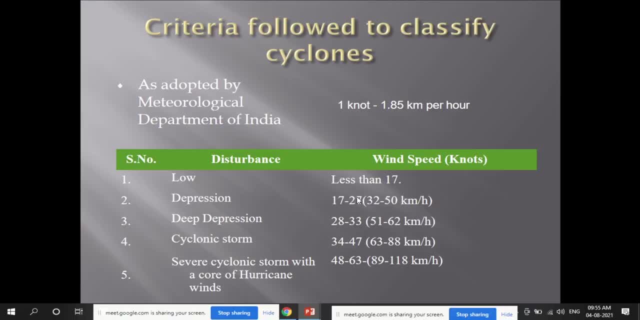 Okay, So how fast? So when the wind speed is less than 17 knots? Sorry, Now what is 17 knots? 17 knots, So 1 knot is 1.85 kilometer per hour, So this particular unit name is given as 1 knot. 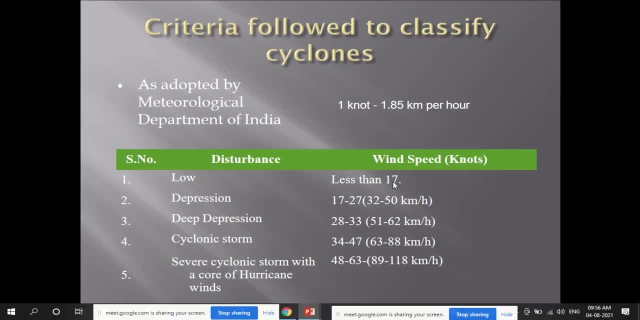 Okay, So when you talk about 1 knot 17.. Okay, So that is around some 32 kilometer per hour. Okay, Depression, That is 70 to 27 knots, That is 32 to 50 kilometer per hour. 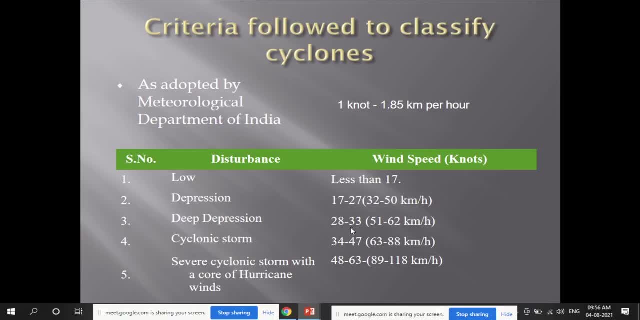 Deep depression: That is 28 to 33 kilometer- I mean knots- That is, 51 to 62 kilometer per hour. Cyclonic storm: That is 34 to 47 knots, Which is around 63 to 88 kilometer per hour. 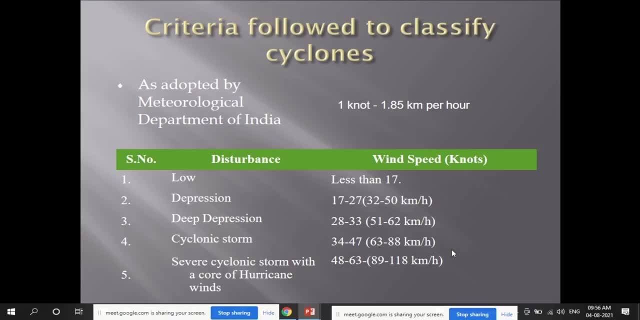 You can calculate also. So 1 knot is 1.85 kilometer per hour, So somewhat you will get the value around this. Then severe cyclonic storm with a core of hurricane winds, So that is 48 to 63 knots. 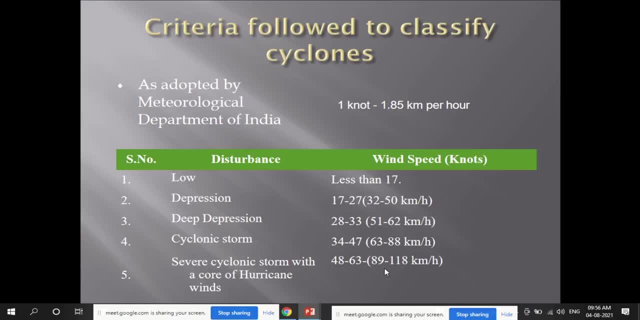 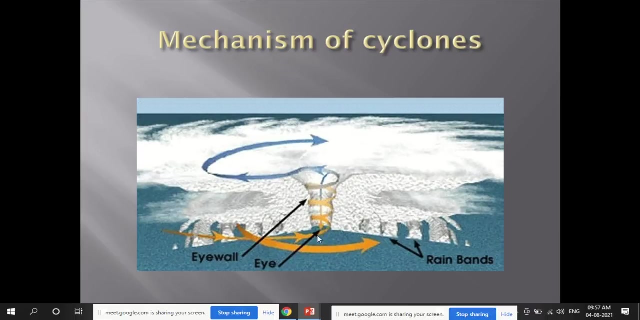 Which comes around 89 to 118 kilometer per hour. So, depending upon the wind speed, the disturbance or the type and the criteria for classification of this cyclone, is done. Then mechanism of cyclone. So, like I told you, in the cyclone the middle part, okay, is a low pressure zone. 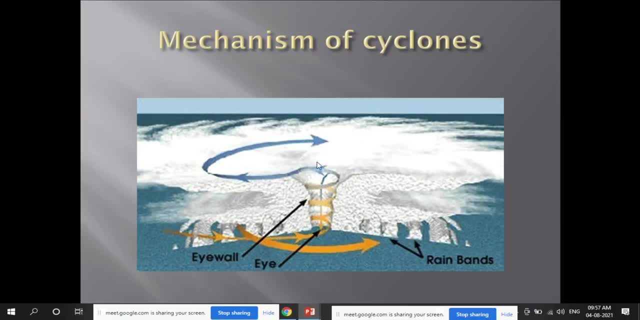 And the outer part where the wind is blowing. okay, in the clockwise or anticlockwise direction, that is, in the high pressure zone. Okay, So the eye is the center part. Okay, The eye wall is the side wall that is formed in that particular cyclone. 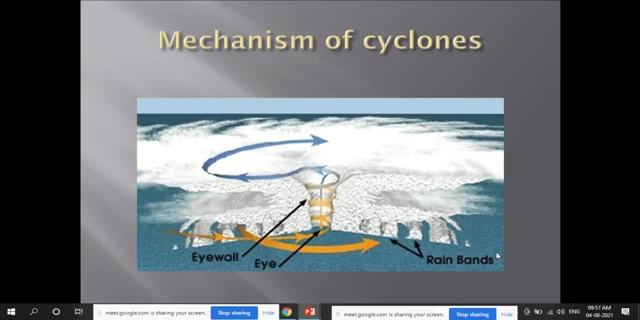 And the rain bands? okay, and the rain bands because of the, because when the cyclone arises inside, it arises inside the water, right, Okay, Because the water, whenever there is, you know, the water gets warm, correct? 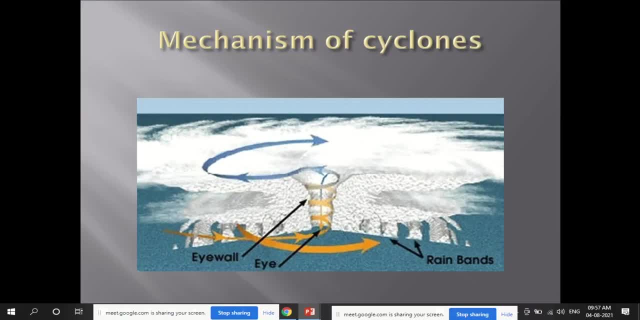 Because of the sun rays And since, at warm area, the low pressure is generated Because of the warming of the water, The water vapors are released, which forms the clouds. Correct, And that's what the- because it's a low pressure zone created. when the water gets warm, this water vapor is created. 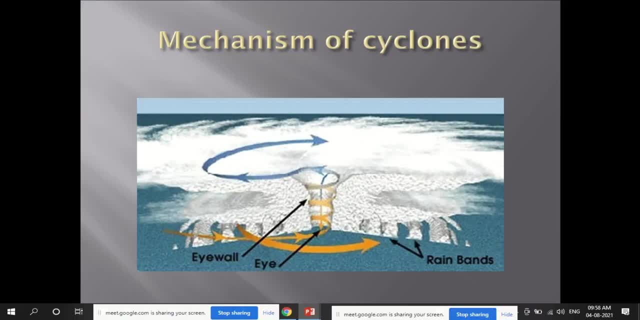 Correct And that is why the low pressure zone is formed at the center And the strong winds okay, which are cooler winds, okay, at high pressure zone, they have high pressure. When there is cooler winds, like cool temperature, there is high temperature. 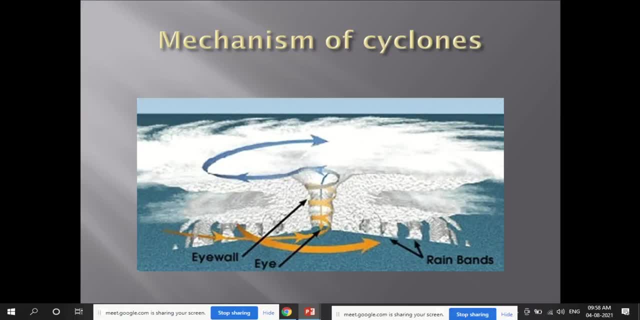 And wind always flows from high pressure to low pressure And that is why the wind from the high pressure zone, where there is cooler atmosphere, they will come and circulate this low pressure area, because here the water vapor form is the warm area, low pressure area. okay. 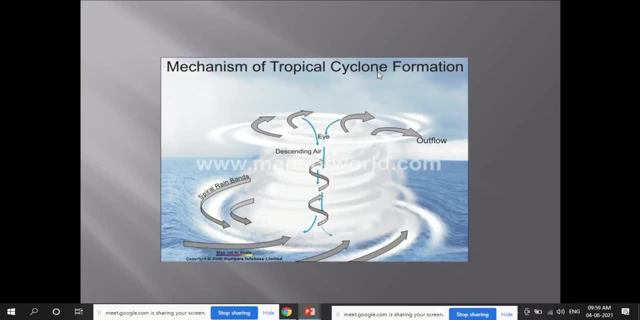 So see here, mechanism of tropical cyclone formation. Now, here you see, See the descending air. If you see this blue arrows, this is air, Because air, like I told you, it flows. that is air or wind flows from high pressure zone to low pressure zone. 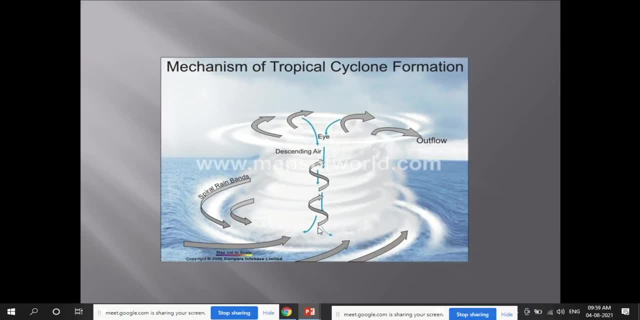 When the middle part- what you see is I is inside- the is in the low pressure zone because it is on the water surface which is warmer, And where it is warm it is low pressure zone, And the and the cooler wind which is, will be in the high pressure zone. 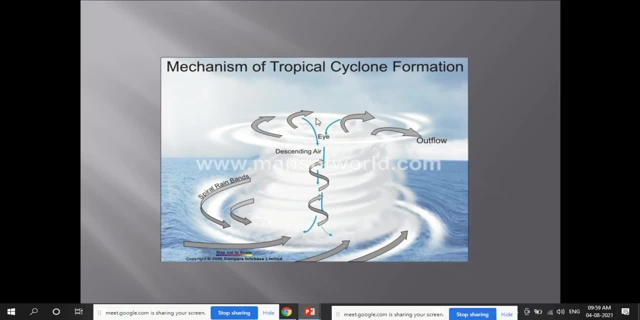 Okay, They will descend because wind will flow from high pressure to low pressure And therefore, you can see the wind blowing inside and descending air. what you see, Okay, And these are the spiral rain bands. Okay, That are flowing outwards. 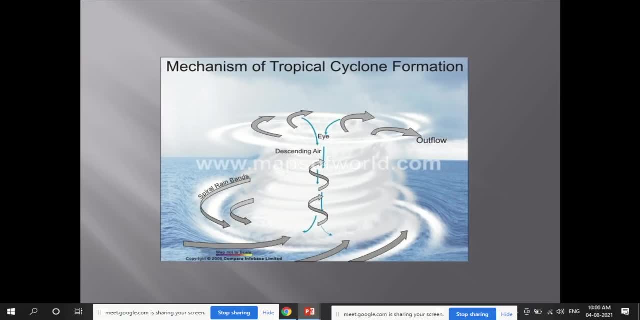 Okay, So this is how the cyclone looks like. Okay, So it's not just the wind, It is the rain band that you see That are formed because of the wind. Okay, Then, mechanism of the cyclone. 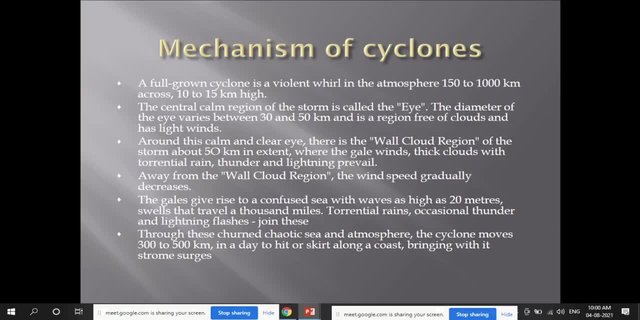 A full grown cyclone is a violent whirl in the atmosphere. 152,000 km across- that is width, And 10 to 15 km high, So it is that violent. The central calm region of the storm is called the I. 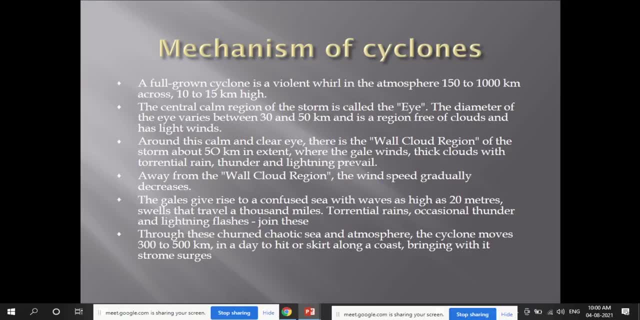 The central low pressure warm region- calm region- is called the I. The diameter of the I varies from 30 to 40. So it is about 50 km And is a region free of clouds and has light winds. Around this calm and clear I there is wall cloud region of the storm about 50 km in extent. 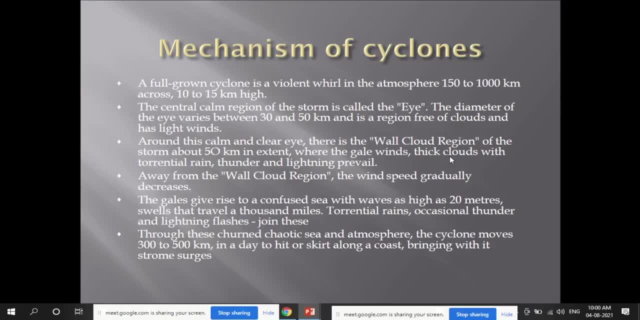 Where this gale winds, the strong winds, thick clouds with torrential rain, thunder and lightning prevail. So around that I is the I wall, which is this combination of this: strong winds, thick clouds, torrential rain, thunder, lightning, etc. 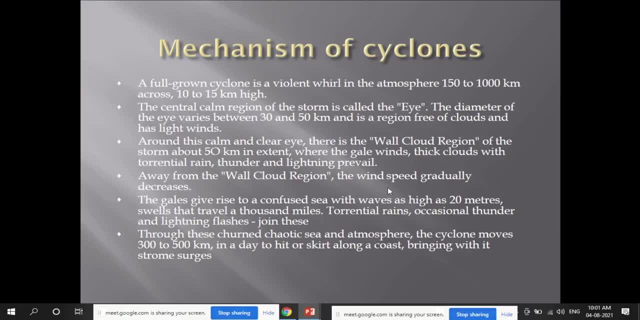 Okay, Away from the wall cloud region, the wind speed gradually decreases. Okay, It is only in the cyclone. that is, the wall cloud region, where the wind speed is more And it gradually decreases. outside, away from the I, The gales give rise to confused sea, with waves as high as 20 meters. 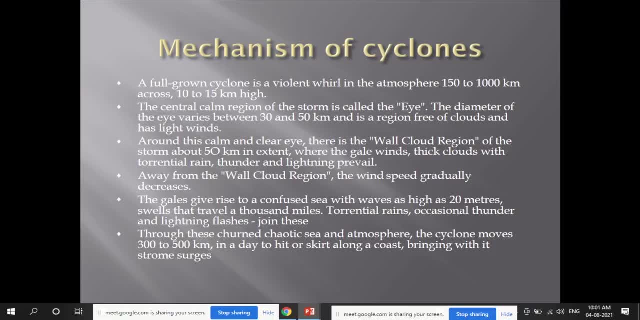 Because of the strong winds. it is the waves that we see getting disturbed, And you know they rises. Okay, So this gale, that is, the strong wind, give rise to confused sea, with waves as high as 20 meters. 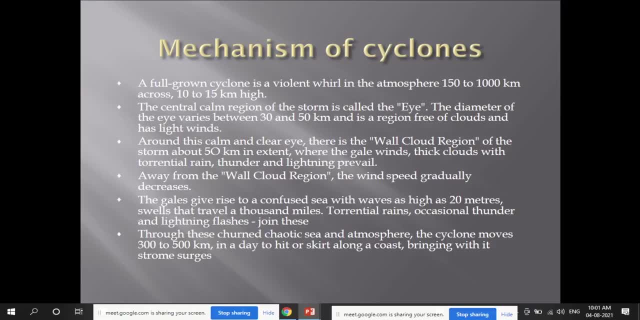 It swells the traveled thousand miles. Torrential rains, occasional thunder, lightning flashes- all this join this particular cyclone. Through this stern chaotic sea and atmosphere, the cyclone keeps moving 300 to 500 km in a day To hit and skirt along a coast. Bringing with it storm surges. Storm surges, in the sense, increase in the sea level. Once the cyclone reaches the higher altitudes, they often change their direction. Once there is the higher altitude, they often change their direction and move north and northeast. 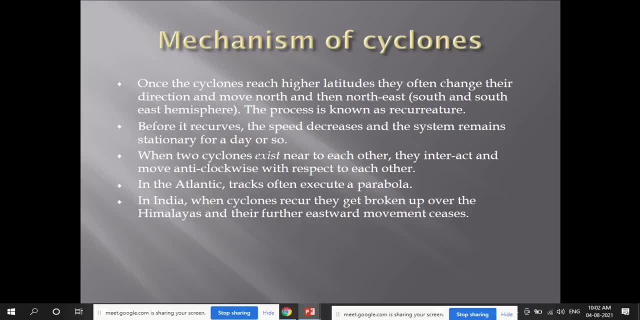 Or when it reaches the higher altitude at the south, it moves south and southeast hemisphere. This process is known as the re-curriature Before it re-curves. Before it re-curves, the speed decreases and system remains stationary for a day or so. 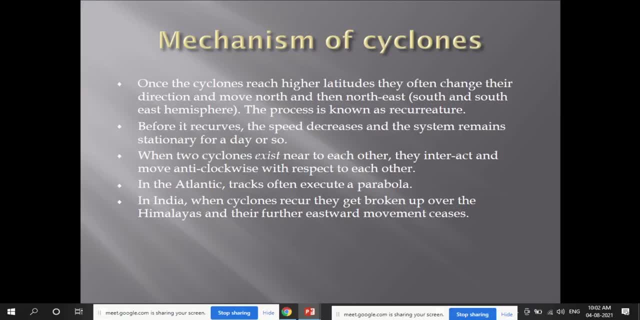 When it reaches the hemisphere. basically, the speed decreases. When two cyclones exist near to each other, they interact and move anti-clockwise with respect to each other. Okay, When this? when there are two cyclones which come near to each other. 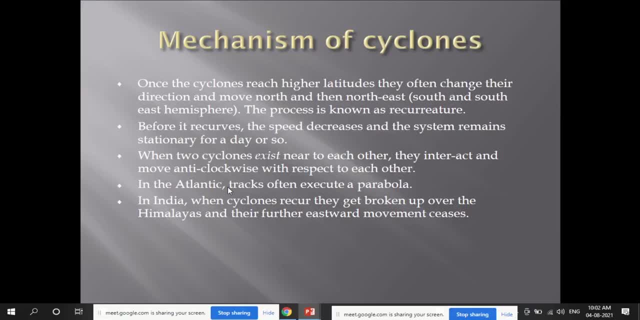 Okay, They move anti-clockwise to each other In the Atlantic tracks often execute parabola, So this interaction often forms like a parabola In India when cyclones re-curve, When this re-curvation happens. 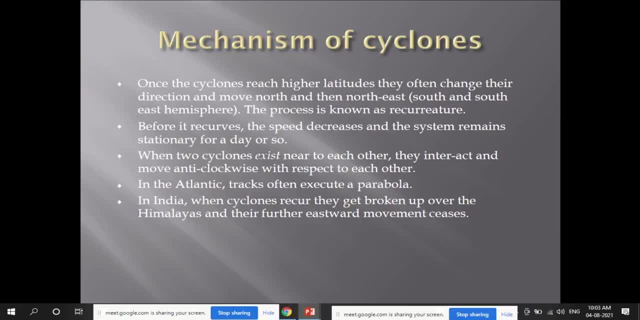 When it reaches the hemisphere, The higher altitude happens. When the cyclones re-curve, they get broken up over the Himalayas, The colder regions, Okay, Higher altitude regions, And their further eastward movement ceases. That is stops. 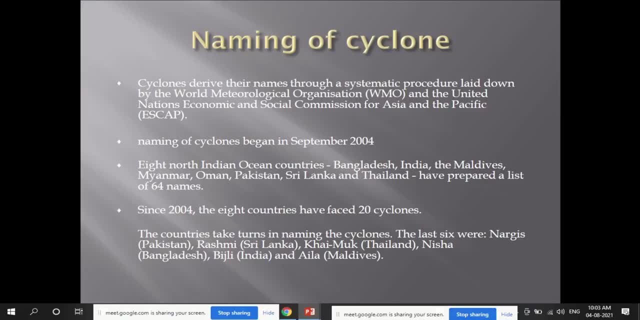 The naming of the cyclone. As you know, every cyclone has some different, different name, Correct. So we have experienced the Nisar cyclone. also, We have just seen the Tope cyclone, also Correct, So this naming is given. 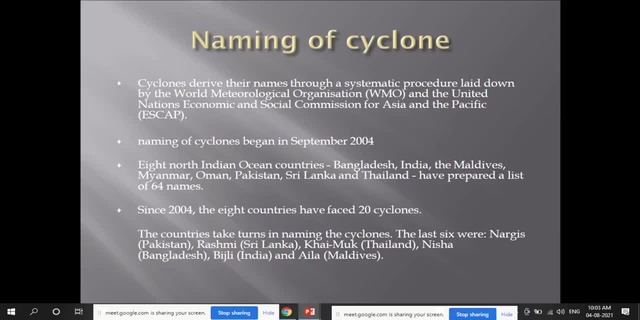 Cyclones derive their names through a systematic procedure laid down by the World Meteorological Organization and the United Nations Economic and Social Commission for Asia and Pacific. Okay, So now you know How these cyclones derive their names, from Which procedure given by WMO and ESCAP. 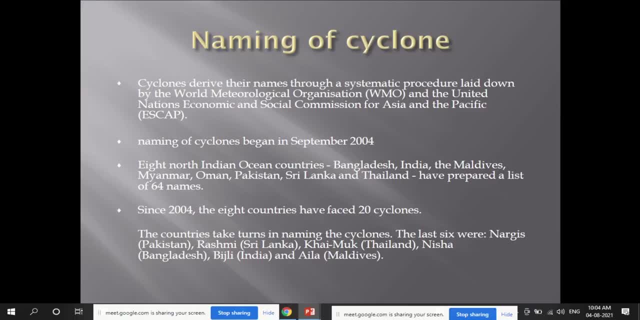 Naming of the cyclones began in September 2004.. 8 North Indian Ocean countries, ie Bangladesh, India, Mayadeus, Myanmar, Oman, Pakistan, Sri Lanka and Thailand, have prepared a list of 64 names. Since 2004,, the 8 countries have faced around 20 cyclones and more than they have experienced in last 2-3 years as well. 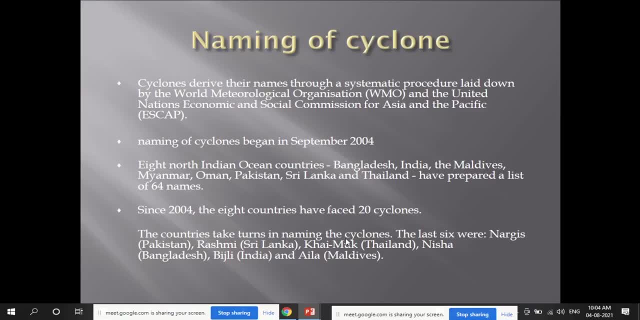 The countries take turns in naming the cyclones. So these 8 countries take turns in naming the cyclones. The last 6, I mean few of them- are Nargis that is named by Pakistan, Rashmi that is named by Sri Lanka, Khai Mook by Thailand, Nisha by Bangladesh, Bijli by India, Ayla by Mayadeus, and many more that we have just seen. 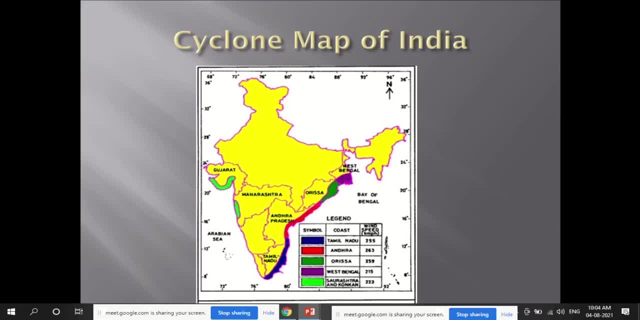 Now, this is the cyclone map of India. Okay, So you can see the wind speed given here. Okay, Tamil Nadu: Basically, the colored areas, apart from the yellow colored areas, are the cyclone prone areas. Okay, And this apart from the yellow part. 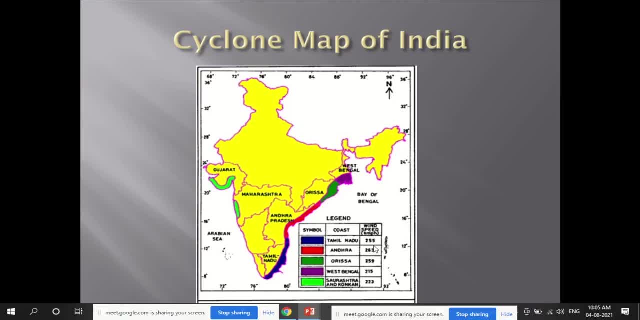 So the blue part, there is Tamil Nadu, where the wind speed is 255 km per hour. The red part, there is the Andhra, Pradesh, Okay, Where the wind speed is 263 km per hour. Okay, This dark green part, which is Orissa. 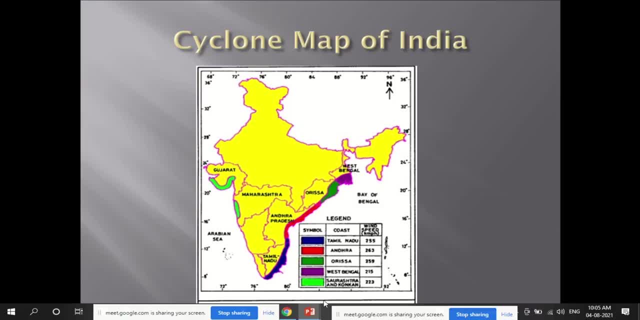 Which is where the wind speed is 259 km per hour. Then this violet or what do you say, purple part, that is, the West Bengal- 215 km per hour, And the light green part, Saurashtra and Konkan, that is 223 km per hour, is the mostly the wind speed in this area areas. 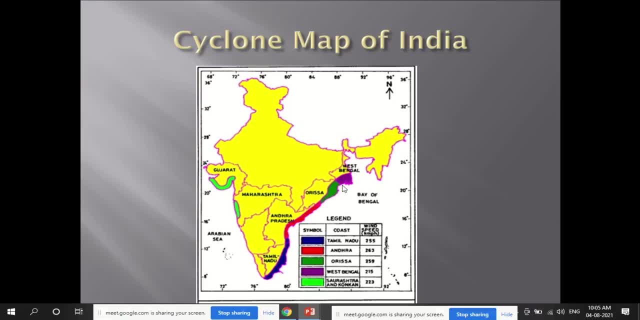 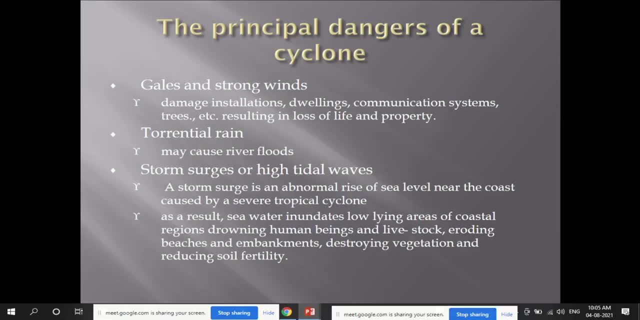 Okay, And these are the cyclone prone areas of our country. Then what are the principal dangers of a cyclone? Gales and strong winds. Gales, that means the strong winds, Okay, Damage: It damages the installations, buildings, communication system, trees, etc. 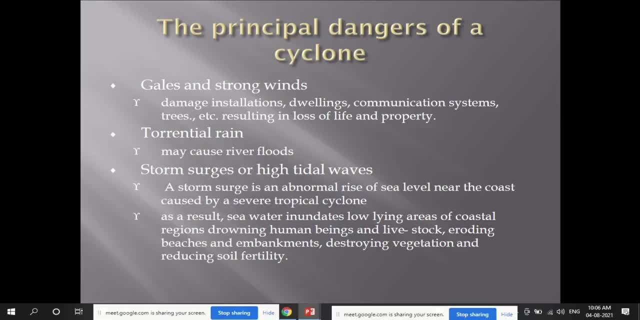 Resulting in loss of life and property. Torrential rains: Too much of rains that causes river floods. I mean the rains associated with these cyclones: Storm surges and or high tidal waves. Storm surges also means when there is increase in the height of the sea. 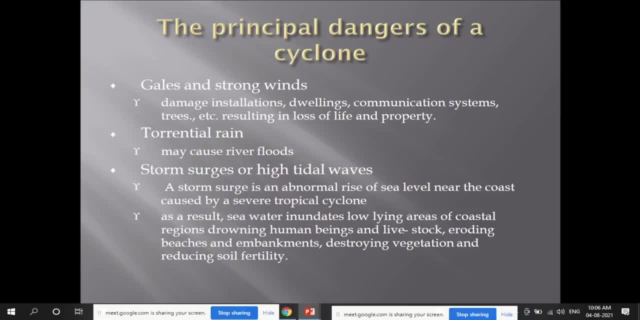 That is for the high tidal waves. A storm surge is an abnormal increase of sea level near the coast caused by severe tropical cyclone. As a result, sea water inundates, that is, comes inside the low-lying areas of coastal regions, Drowning the human beings and the livestock, the animals, eroding beaches and embankments, destroying vegetation and reducing the soil fertility. 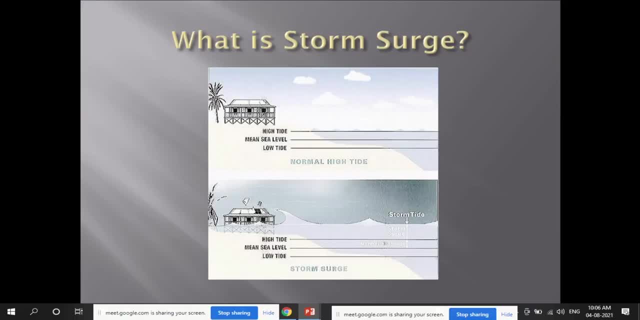 So these are the principal dangers of a cyclone. So now you will see in this picture what is a storm surge. When there is a normal high tide, Okay Means sea level low tide and high tide, But when there is a storm surge because of the cyclonic action, the sea waves rise above this high tide. 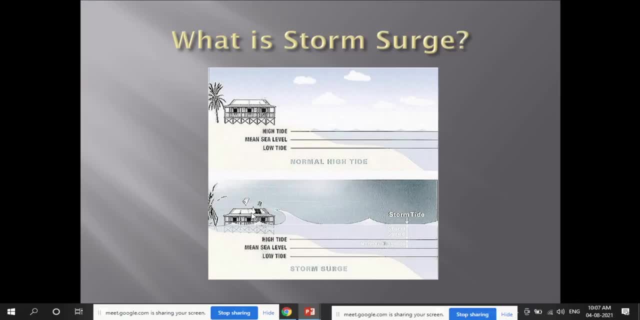 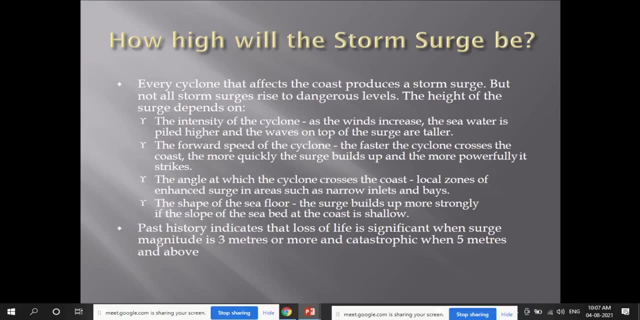 See this Storm, tide, Okay, And damaging properties, Then how high will the storm surge be? Every cyclone that affects the coast produces a storm surge- Okay, Increases the sea level, But not all storm surges rises to dangerous level. 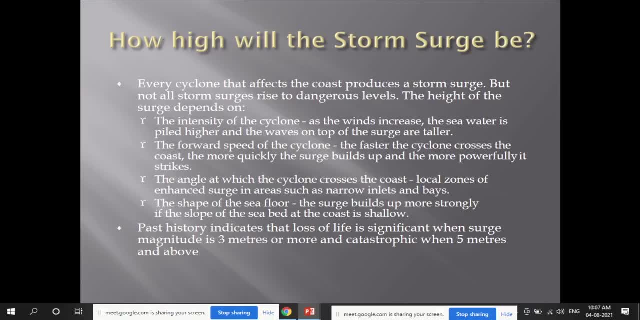 The height of the surge depends upon the intensity of the cyclone. As the wind increases, the sea water is piled higher and the waves on top of the surge are taller. Okay, More the intensity. Okay, More, the higher will be the storm surge. 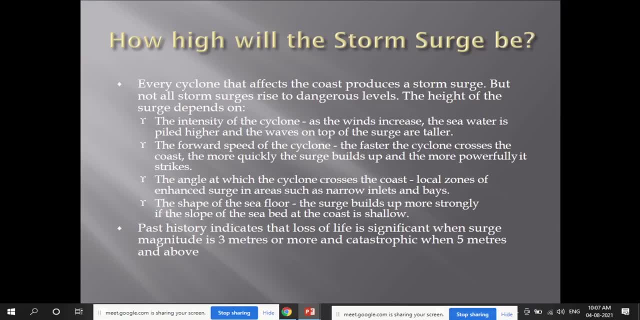 The forward speed of the cyclone. The faster the cyclone crosses the coast, the more quickly surge builds up And more powerfully it strikes. The more near- I mean when cyclone travels- Okay, If it crosses the coast with higher speed, the more will be the increase in the sea level near the coast. 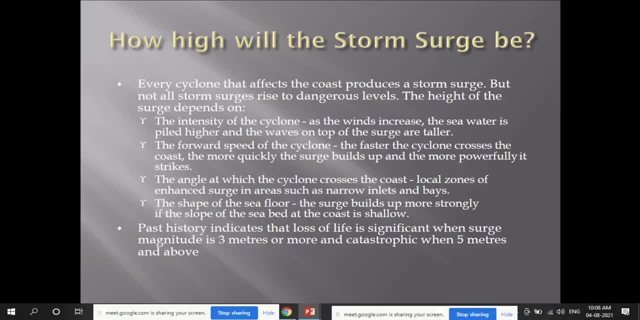 Of course, The angle at which the cyclone crosses the coast, Local zones of enhanced surge in areas such as narrow inlets and bays. That is also one of the reason. That is intensity, The forward speed of the cyclone with which it arises the coast. 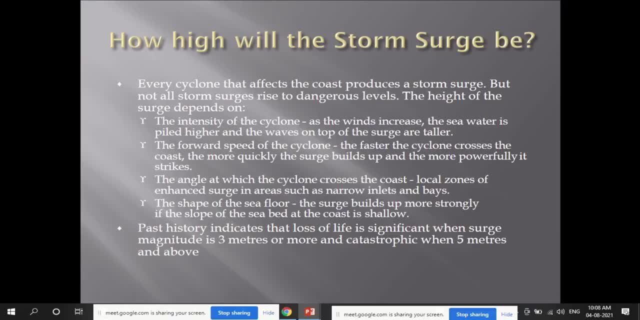 Angle at which the cyclone crosses. Okay, These are the reasons that how much the rise in the sea level will be, Then shape of the sea floor Surge builds up more strongly if the slope of the sea bed at the coast is shallow. 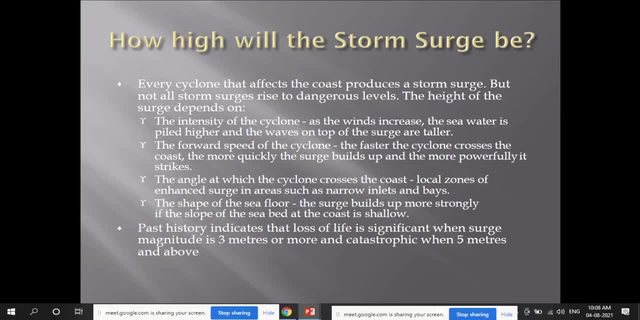 So, of course, when near the sea bed the depth of the sea is low, That is, shallow, The storm surge will build in that particular area. Past history indicates that loss of light is significant when surge magnitude is 3 meters or more. 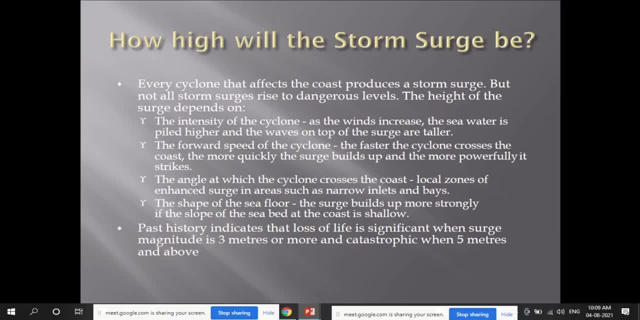 Okay, You have seen the diagram now. High tide level is one level And above that is the storm surge Increasing the sea level. If the magnitude is more than 3 meters, it is dangerous condition, Okay, But when it is more than 5 meters, 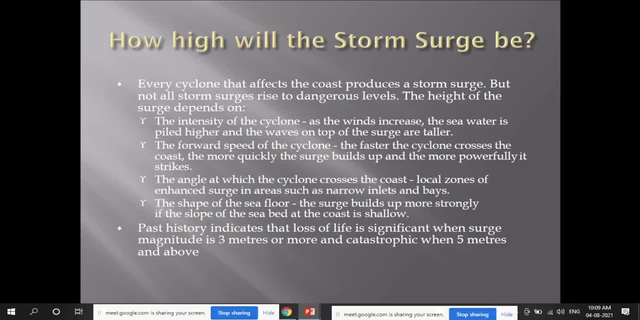 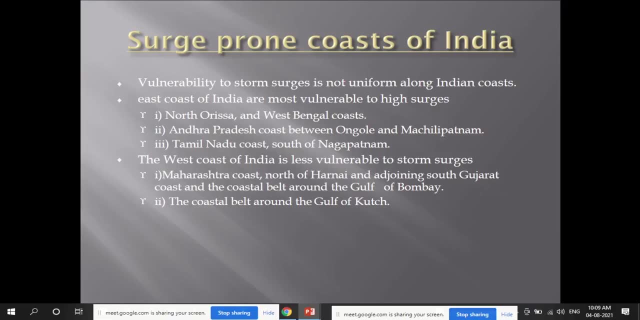 It is catastrophic Deadly condition Surge from coast of India. Vulnerability to storm surges is not uniform around the Indian coast. Right East coast of India are most vulnerable to high surges. That is, the North Orissa, West Bengal coast. 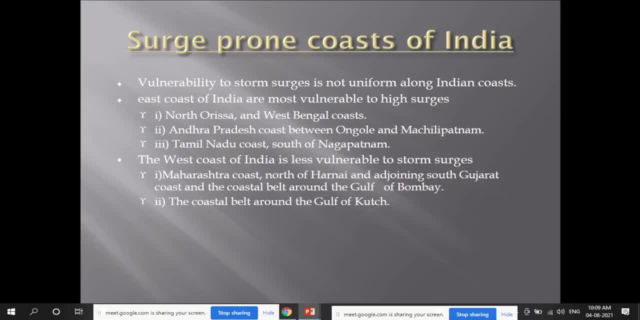 Andhra Pradesh coast. Coast between Angol and Machinipatnam. Tamil Nadu coast South of Nagapatnam. The West coast of India is most vulnerable. The West coast of India is less vulnerable to storm surges. Okay, Storm surges. 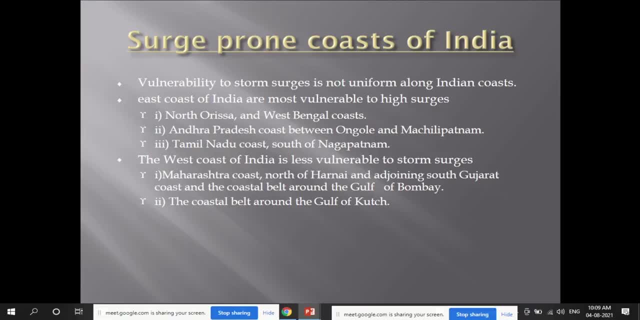 That is, increase in the sea level, Higher increase. So that is West coast of India is less vulnerable to storm surges. That is Maharashtra coast North of Harnai and adjoining South Gujarat coast And the coast bed around the Gulf of Bombay. 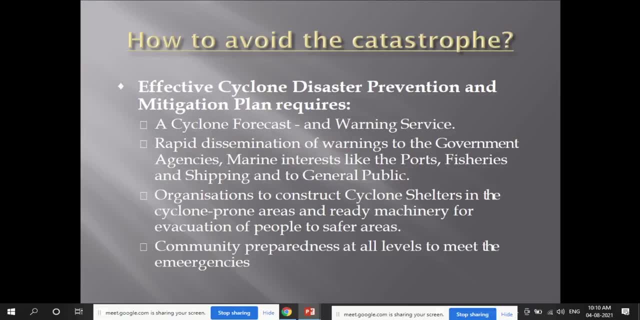 The coastal bed around the Gulf of Kutch. Okay, Then, how to avoid the catastrophe. So effective cyclone disaster prevention and mitigation plan is required to avoid this particular disaster, A cyclone forecast and warning service that now we usually get it. 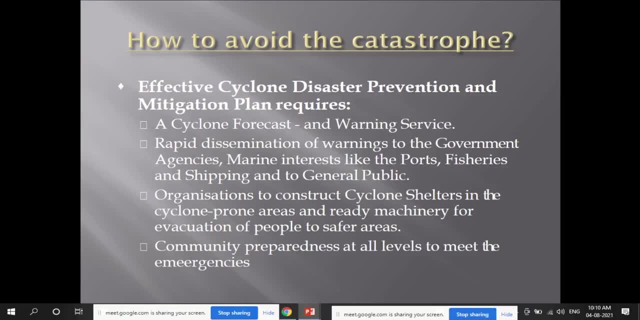 Rapid dissemination, that is, spreading of warnings to the government agencies, marine interest, like the ports, fisheries, shipping- and to the general public, Specifically more to the people which are dependent on the sea and which live near the sea- They have to be informed very prior- and also to the general public. 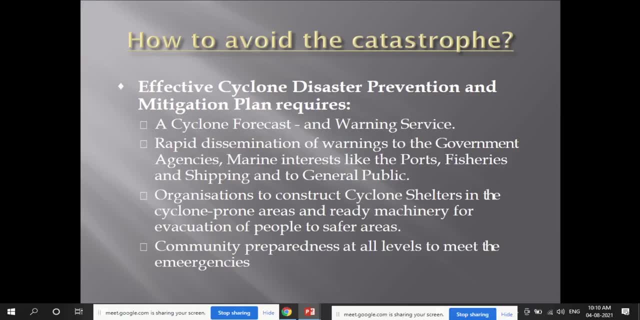 Organizations to construct cyclone shelters in the cyclone prone areas and ready machinery for evacuation of the people to safer areas. As you know, when there is cyclone and the storm surge and everything, most important thing when you get the early warning sign is evacuation of those people from that cyclone. 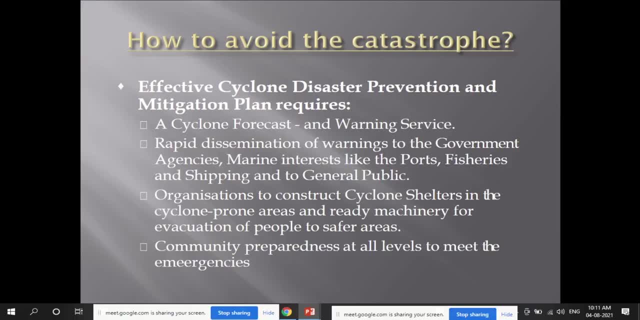 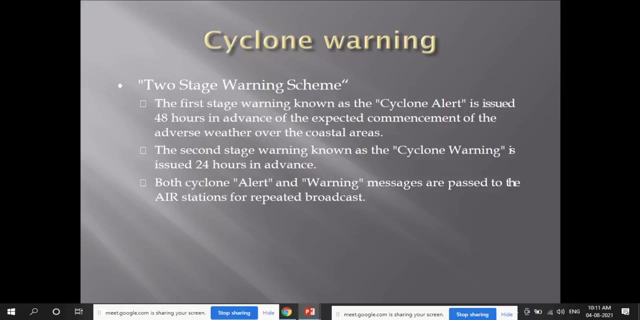 prone areas. Okay, Thank you. Bye, Bye, Bye, Bye, Bye, Bye, Bye. All right, So glad that I think it is going in the form of how to evade the cyclone corners and the expected commencement of the around the. 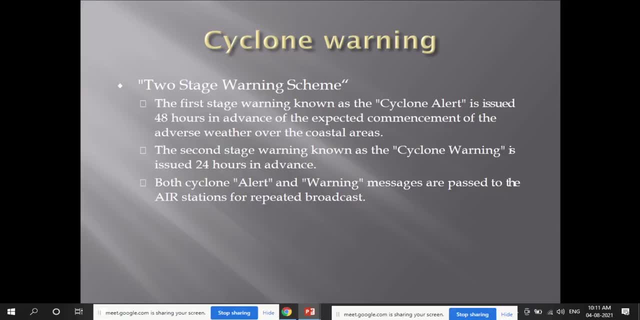 commencement of the adverse weather over the coastal areas. Okay, that is called the cyclone alert, 48 hours in advance to the commencement of such a weather. And the second stage warning is known as the cyclone warning, which is issued 24 hours in advance. 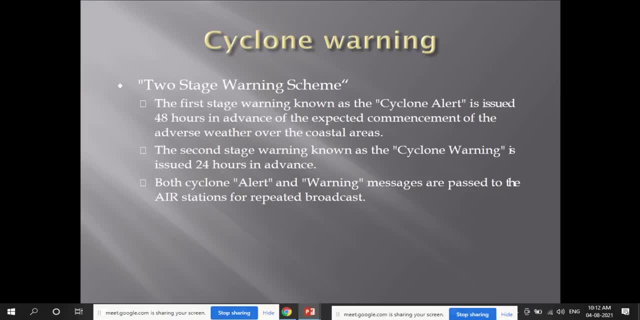 So you have cyclone alert and cyclone warning. Cyclone alert is prior to 48 hours and cyclone warning is issued 24 hours in advance. Both cyclone alert and warning messages are passed to the all India radio stations for repeated broadcast. 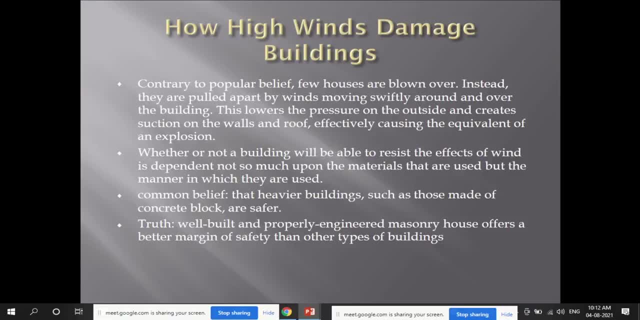 Then how high winds damage the buildings. Okay, so, in short, I will just tell you how this high winds, because of the cyclone, damage the buildings. So, contrary to popular belief, few houses are blown over. Instead, they are pulled apart by winds moving swiftly. 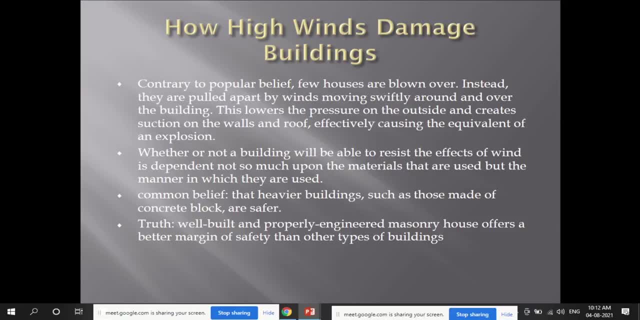 around the buildings. This lowers the pressure on the outside and creates a suction on the walls and roof, effectively causing the equivalent of an explosion. Whether or not a building will be able to resist the effect of the wind is dependent not so much upon the material. 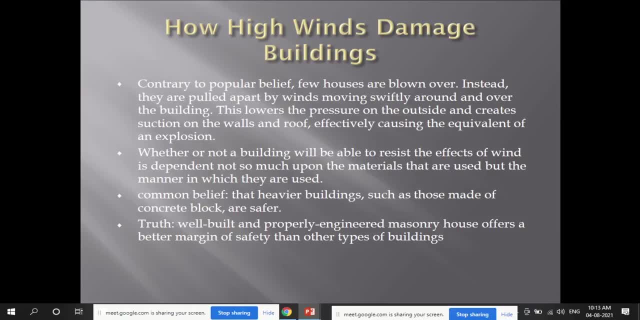 that are used. but the manner in which they are used, Common belief is the heavier the building, such as those made of concrete blocks, are safer. Correct, it is a common belief that whenever there are strong winds, if the construction is of a higher material, a high weight material, 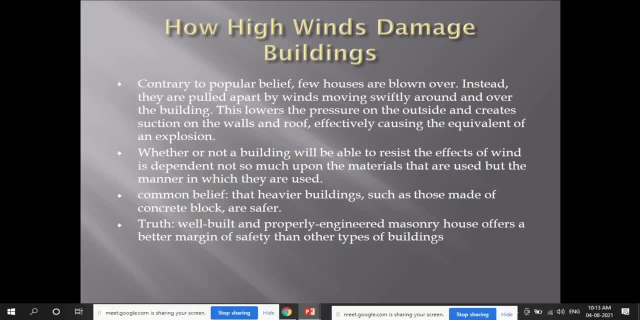 Okay, so it is not. it is safe, We say, but the truth is. well built and properly engineered masonry house offers a better margin of safety than other type of building. It's not just a material, It's a myth that only material is responsible to deal with. 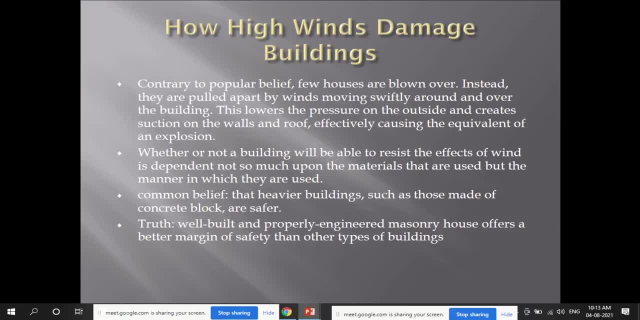 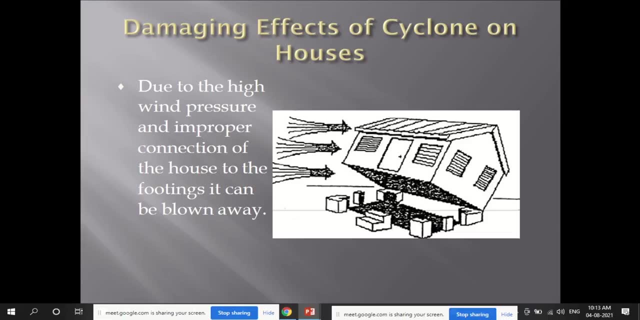 this wind. It is how you construct, how engineered practices are followed in order to deal with such high winds. See damaging effects of cyclone on houses. due to high wind pressure and improper connection of the house to the footing, It can be blown away. 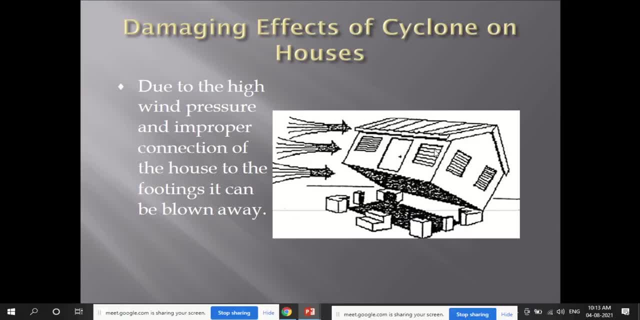 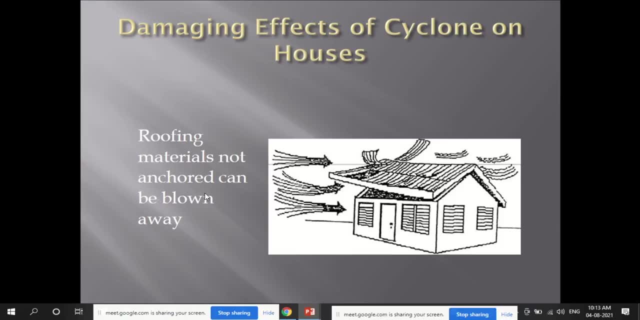 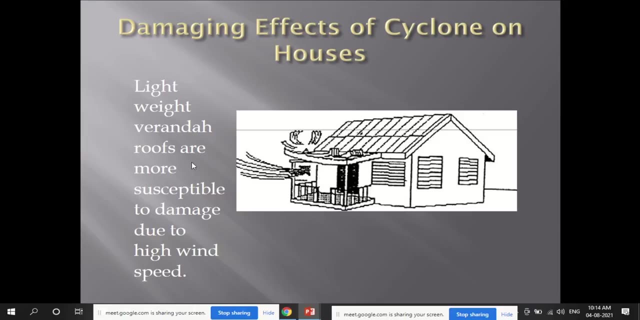 Okay. So what is the use of the construction material that is being used? if it is not proper, connected to the footing, then roofing material not anchored and can be blown away. not properly anchored, lightweight veranda: Okay. veranda roofs are more susceptible to damage. 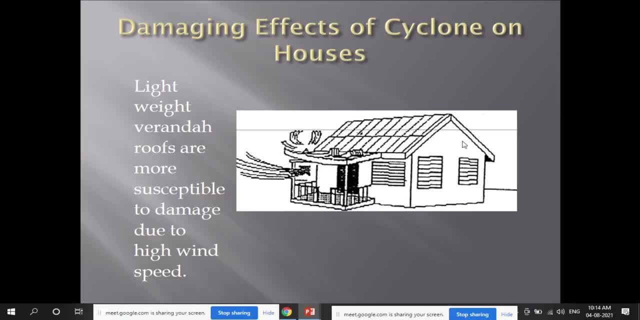 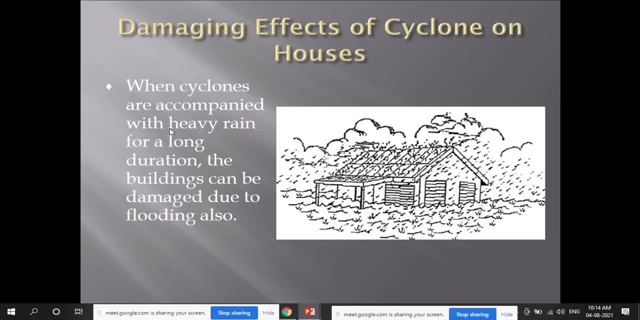 You do high wind speed if the construction material using me in the house is heavier. But what is the use of? the veranda is of lightweight and it is going to get damaged easily. Then, when Cyclones are accompanied with heavy rain for a long duration, the building can be damaged due to flooding. 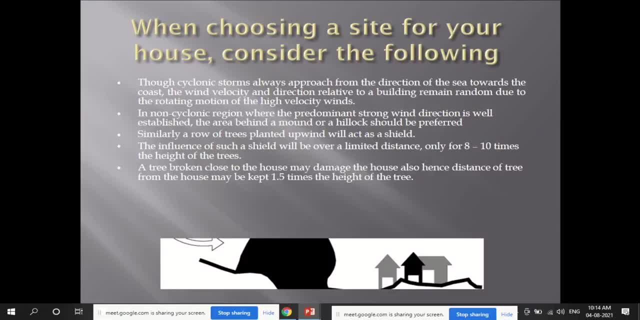 So you know that. so, when choosing the site for your house, consider the following Through: Cyclonic storms always approach from the direction of the sea. Those Cyclonic storms approach from the direction of the sea towards the coast. Wind velocity and direction relative to a building and even. 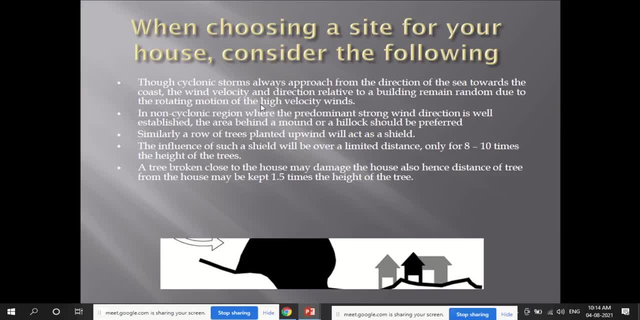 random due to rotating motion of the high-velocity wind Correct. So in non-cyclonic region, where the predominant strong wind direction is well established, the area behind a mount or a hill out should be preferred. In Cyclonic storm, it is not predictable, to it is you cannot predict. 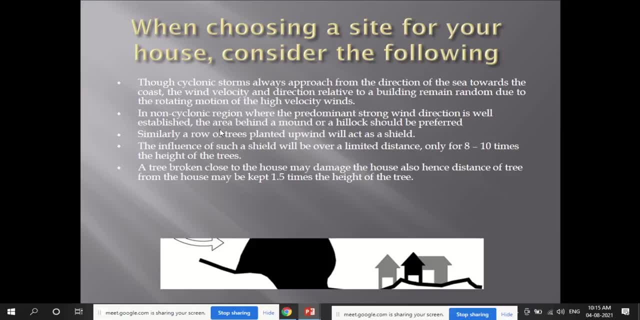 the wind velocity and its direction. But in non-cyclonic region you have the wind direction. So there has you know, it is well established this direction of the wind. So area behind a mount or a hill out should be preferred, Okay. Similarly, a row of trees planted to a wind will act as a shield. 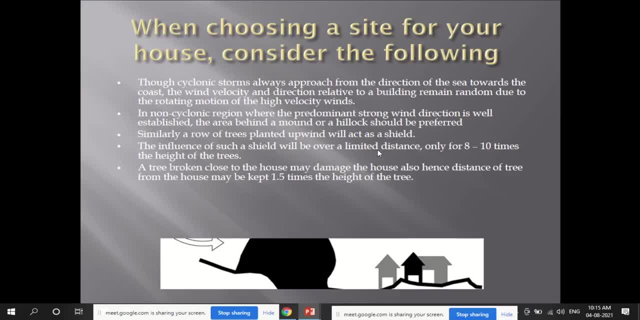 row of trees. Influence of such a shield will be over a limited distance, only 8 to 10 times the height of the wind, Of the trees. Okay, The trees should also not be near to the houses. 8 to 10 times the height of the trees should be the distance between the trees. 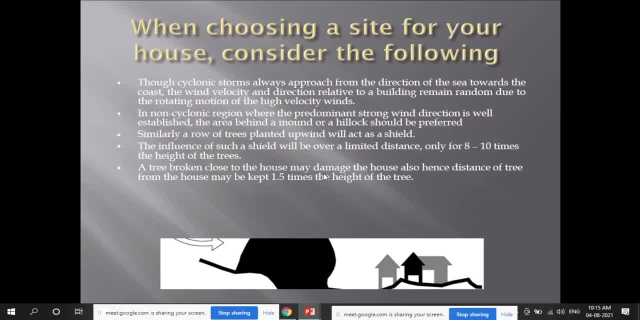 and the houses. A tree broken close to the house may damage the house also. hence the distance of the tree from the house may be kept 1.5 times the height of the tree. Okay, The influence that is of the shield should be 8 to 10 times the. 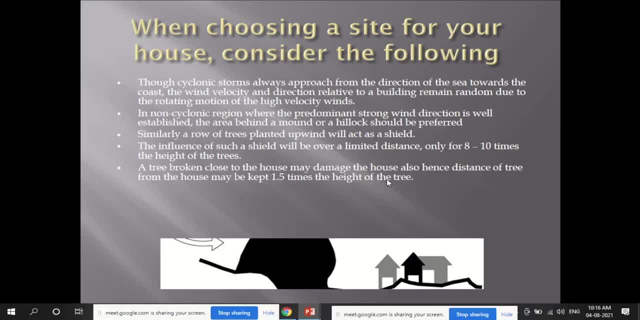 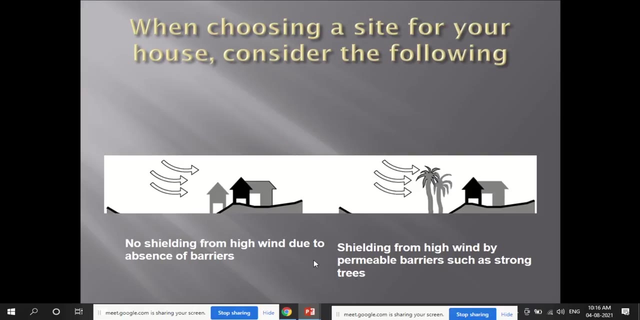 height of the trees And the distance at which the construction to be done should be 1.5 times the height of the tree. See. when choosing the site for your house, consider the following: no shielding from high wind due to absence of barrier and shielding from. 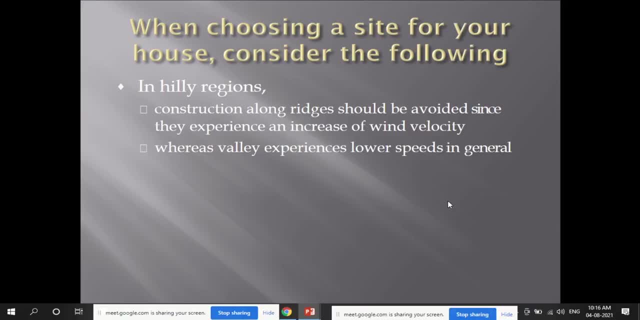 high wind due to these barriers. Okay, Then see here. in hilly areas, construction along the ridges should be avoided. The experience increase in the wind velocity, whereas valley experiences lower speeds in general. So you know that. Okay, See here also. When you have storm surges, the construction should be such that the houses are at higher elevations. Rather than having such a row type arrangement, you should have a cluster arrangement, so that wind could be blocked in all the directions. See these: These roofs could be attached.